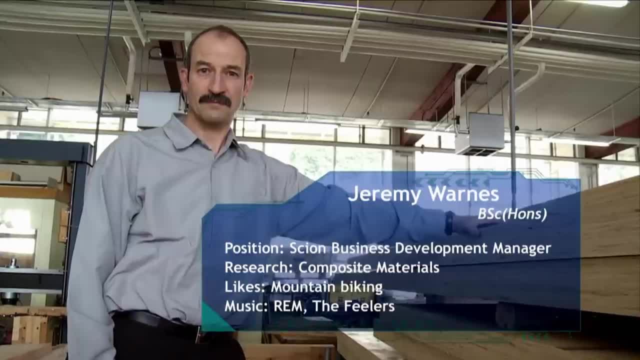 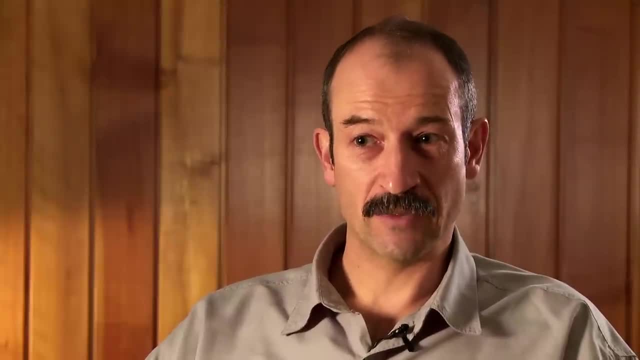 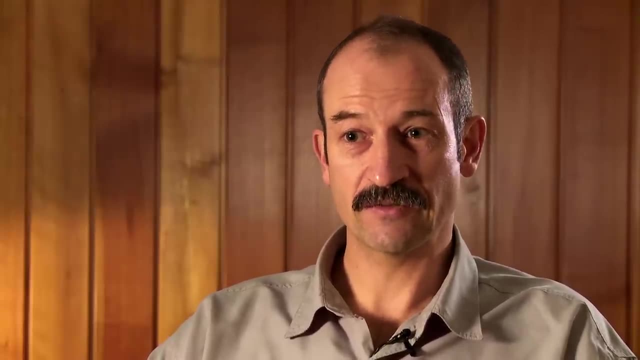 stop tour of how they're trying to replace petrochemicals with green chemistry. Green chemistry is chemistry where there's minimised waste, where there is minimised energy utilisation and also, if you can, from sustainable raw materials you're going to derive the precursors for the chemistry. 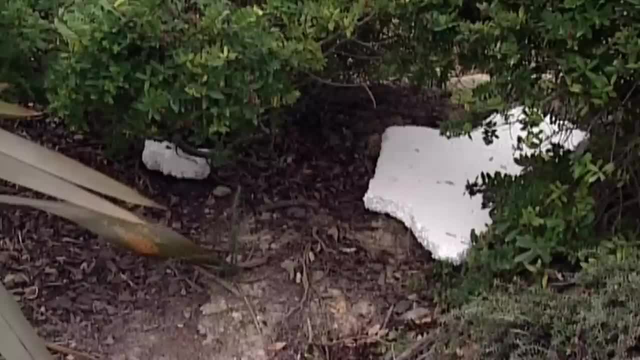 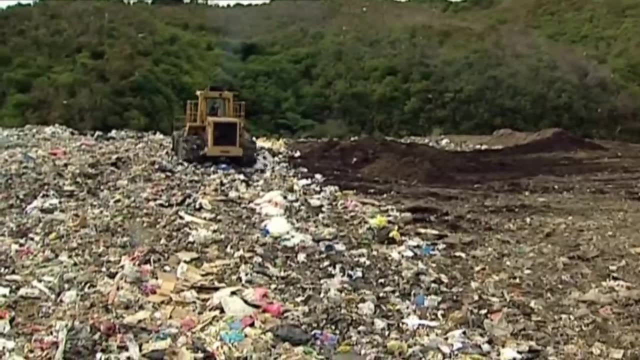 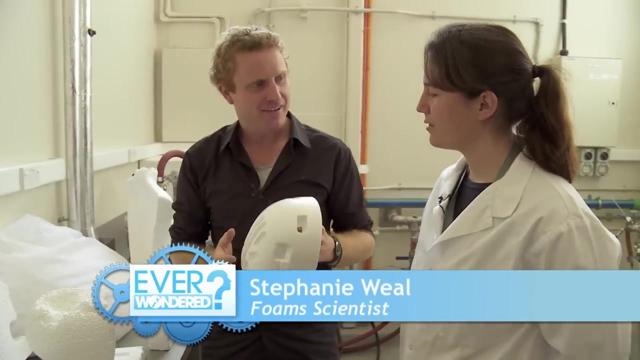 One petrochemical that desperately needs to be replaced is polystyrene. We use this product in unimaginable quantities, but it takes centuries to break down and is environmentally hazardous. Stephanie, what's so special about this helmet? It's made from pyelactic acid. 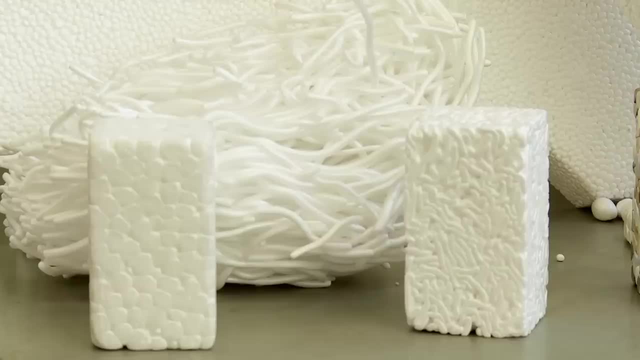 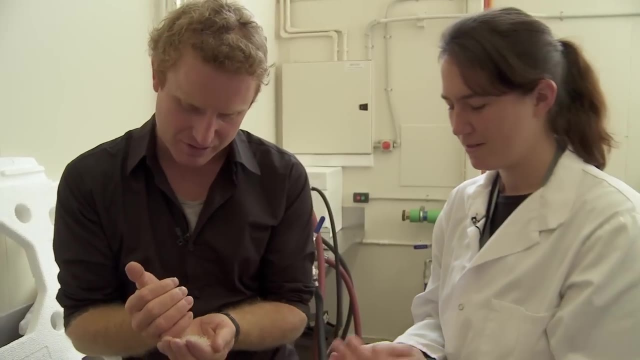 This is bio-derived. Yeah, It's made from corn. This puffy polystyrene started out life as solid little pellets. It looks like plastic, but you say it's from corn. Yeah, no, it's the same behaviour and properties as plastic, it's just that it's sustainable. 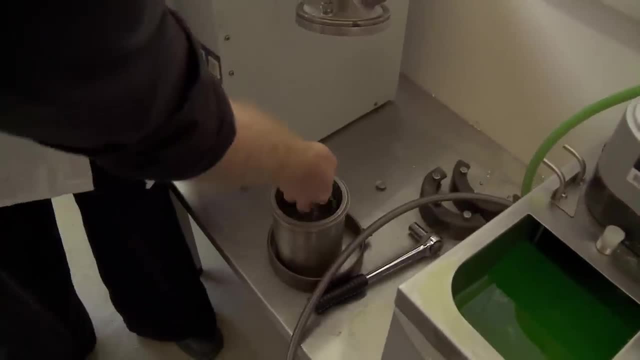 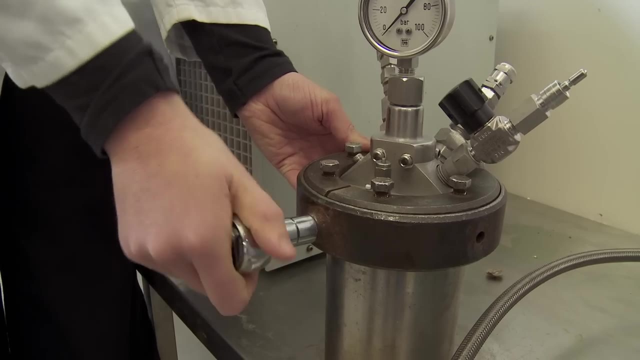 and can be renewable. Corn plastic has been around for a while now, but the problem that Scion has solved is to find a way to puff these little pellets up so that they can be used as polystyrene. The first step is to use hybrids. 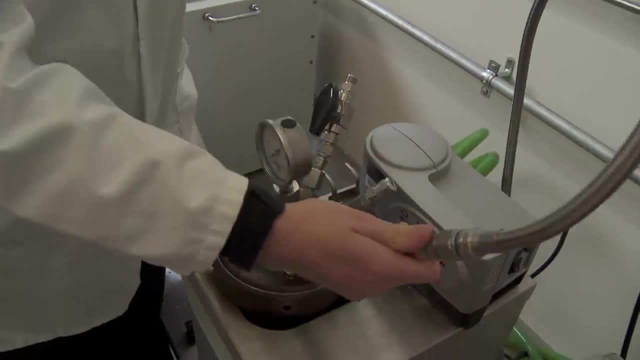 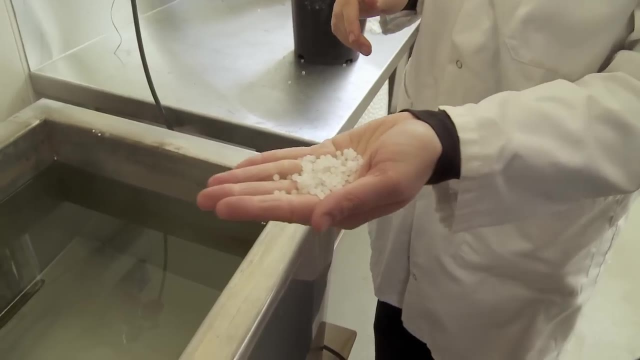 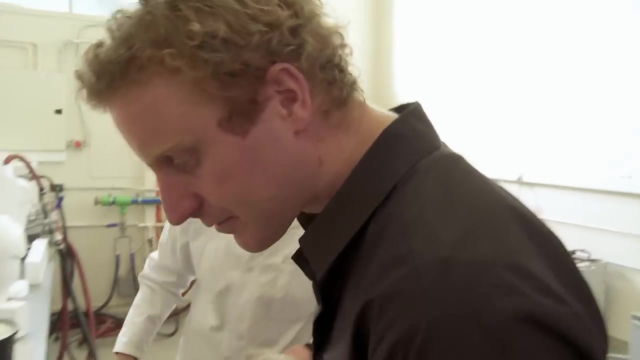 Hybrids are high pressure to force carbon dioxide gas into the solid plastic. That's the CO2 line, is it Yeah? Once this is done, the gas infused pellets are given a nice warm bath. This softens the plastic and allows the carbon dioxide to escape. 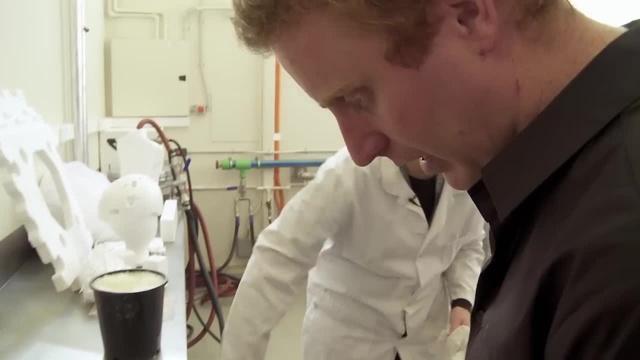 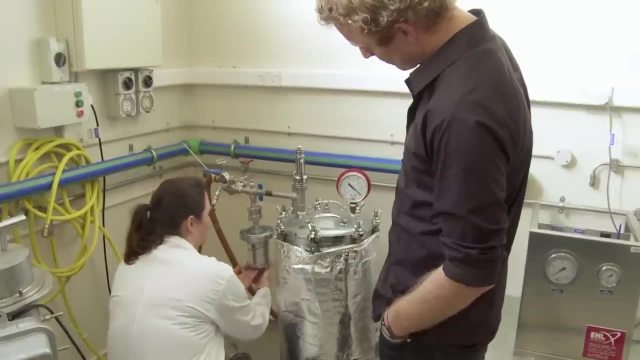 Ah, popcorn. So this is the CO2 coming out and expanding it as it goes. The puffed up bio-plastic can now be shaped into air. So this is the CO2 coming out and expanding it as it goes. The puffed up bio-plastic can now be shaped into air. 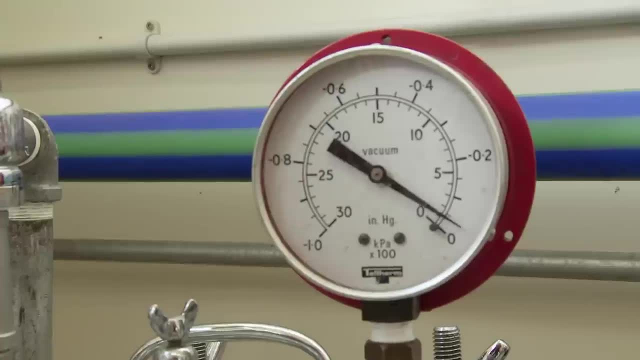 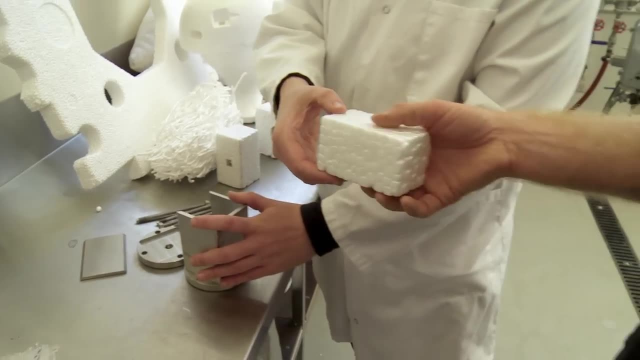 The puffed up bio-plastic can now be shaped into air. It's different from anything that polystyrene can, and Scion are ready to start capturing some of the multi-billion dollar polystyrene market. It's a relatively simple invention, but often some of the best inventions are those that 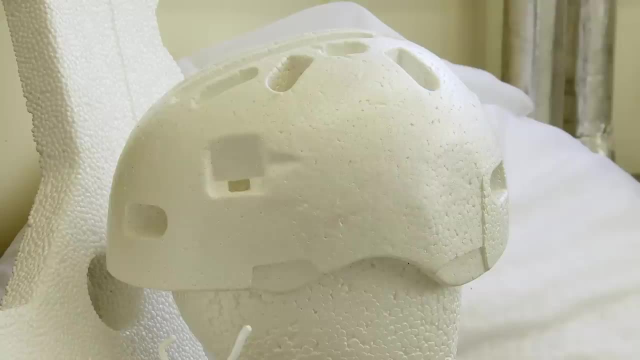 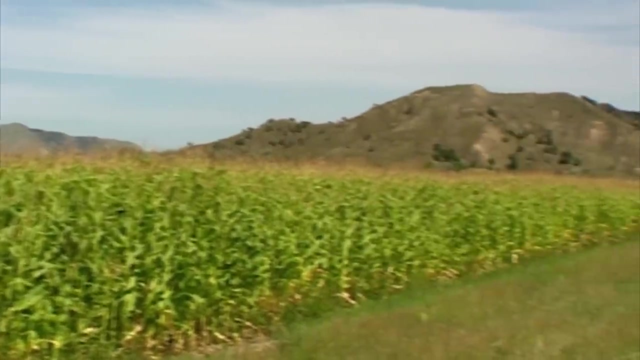 are very simple. We're in that stage now. various companies have tried this technology and hopefully in the near future we'll see some of this product on the market. Making bio-plastic from corn has caused huge controversy because it inflates the price of this food crop that is vital to the survival and health of the environment. 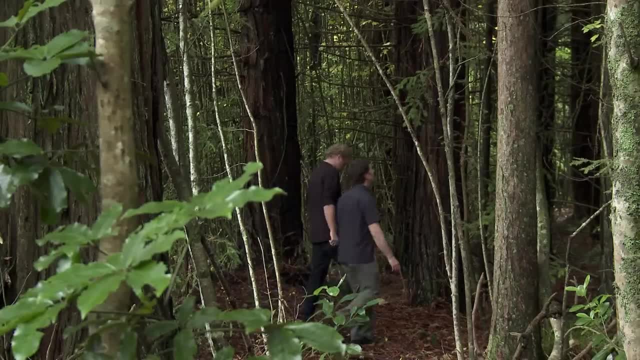 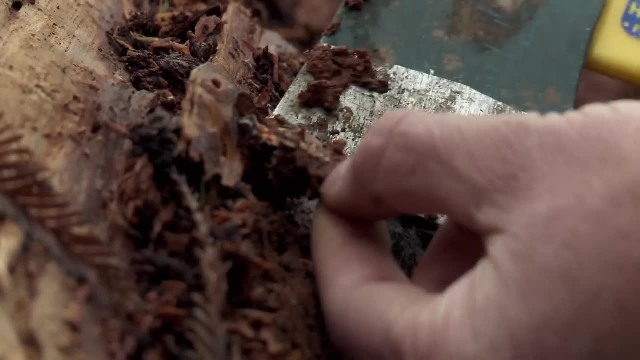 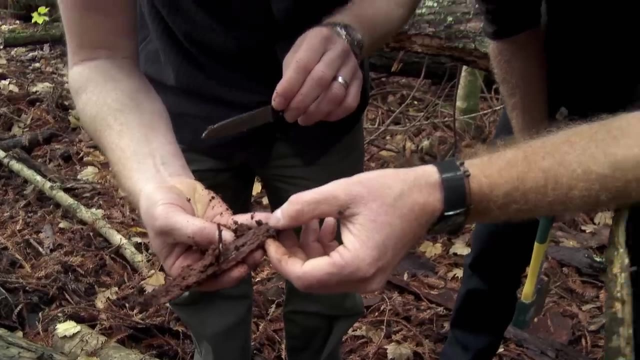 survival of millions. So Scion have recently begun a hugely ambitious project to create plastic from wood. To do this, they have to first break down the wood, So they're studying something that does that already: Termites. To break down the wood, they rely on microbes that are in their guts, So their guts contain 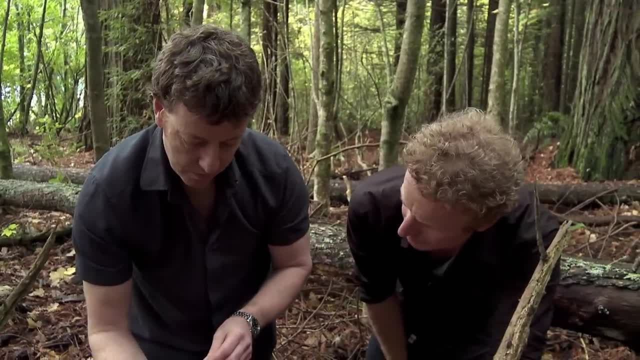 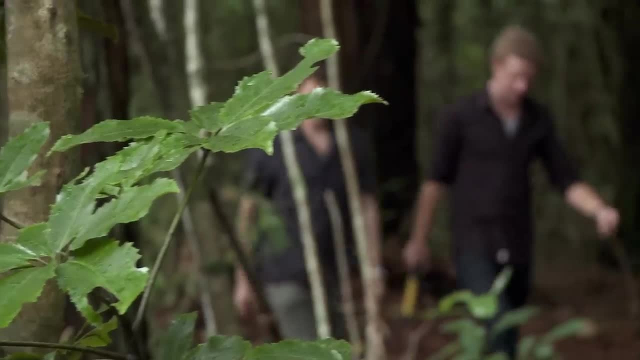 bacteria and protozoa that actually break down the wood, And that's what you're interested in. We're interested in the enzymes that the microbes and the protozoa actually have. Gareth is particularly interested in lignin, which makes up about one third of the tree. 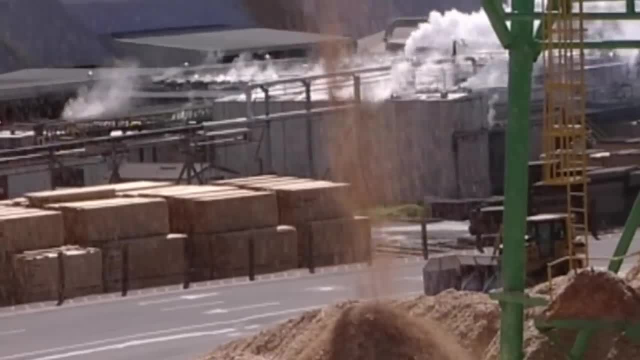 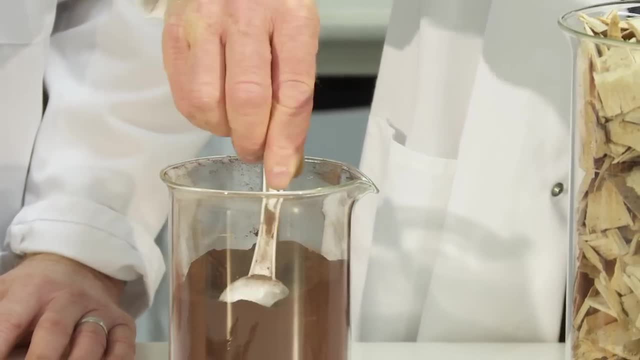 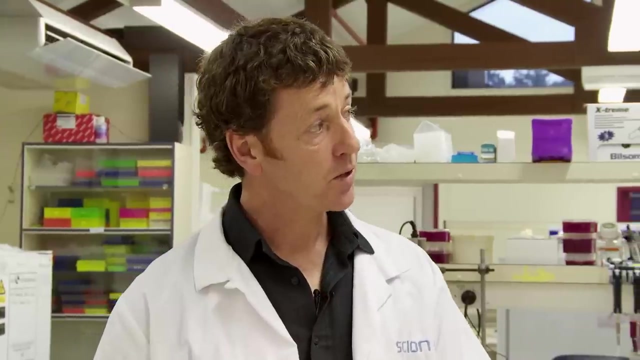 This is a waste product of much wood processing. This leaves a lignin mountain that Scion think that they can mine for global benefit, And what's your kind of vision for this? What do you see it going on to make? We would look at lignin as being a supplier of a lot of the petrochemical source chemicals. 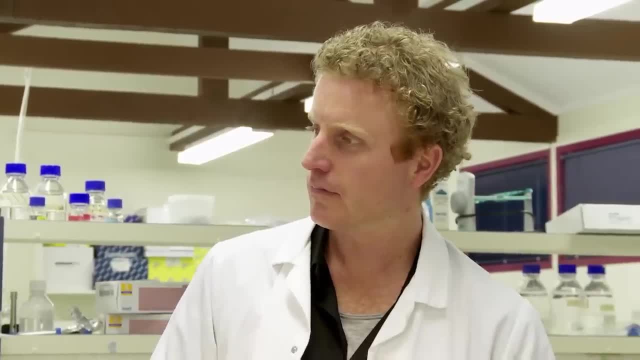 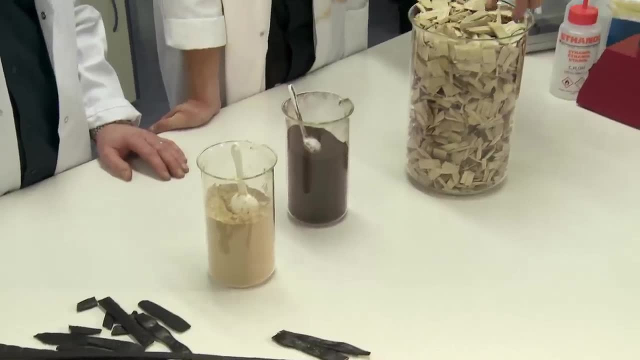 that are currently used in plastic And looking at more sustainably produced plastics that use basically a tree as its starting material rather than a depleting resource such as oil. There is huge value locked away inside the lignin, because it contains many of the same. 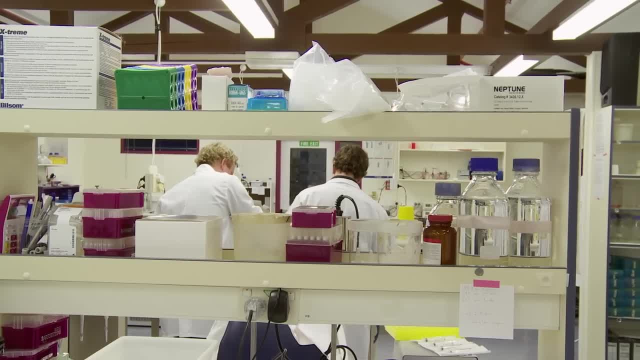 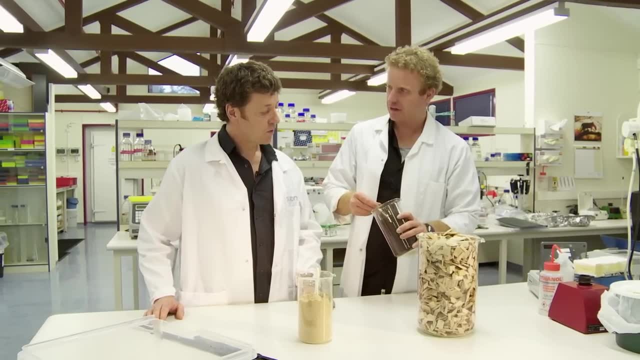 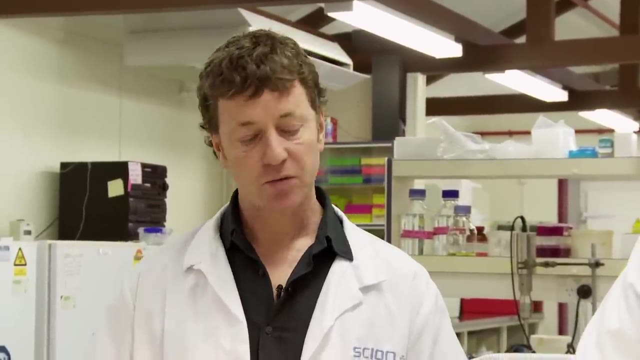 chemical components as oil, But its complex structure makes it very hard to use. So Gareth is identifying how the natural world breaks down the tough lignin. So you're making the lignin much more workable by doing some Making it more workable and expanding the breadth of what it can be used for What we've. 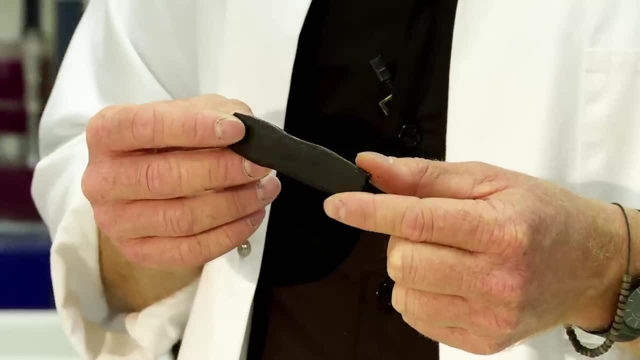 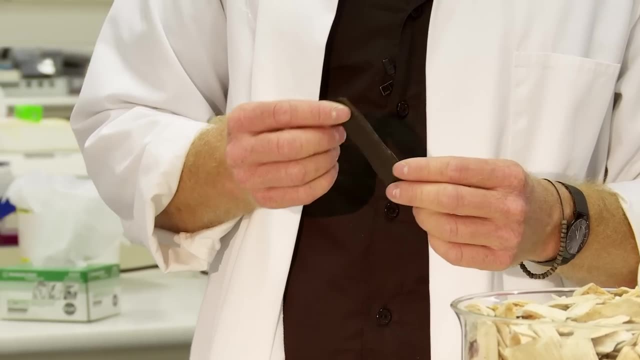 got. here is an example of a lignin and we've extruded it and by melting it has changed quite considerably from this example here. Yeah, so it almost looks like plastic. now It's starting to look very, very plasticky. This is about 70% lignin. It's not very strong. 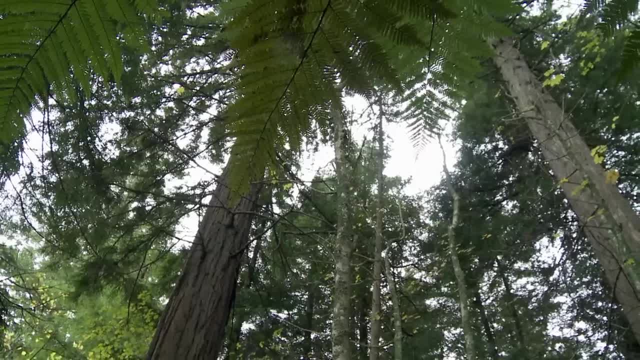 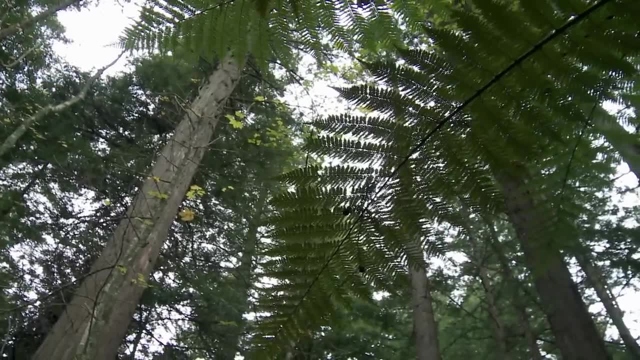 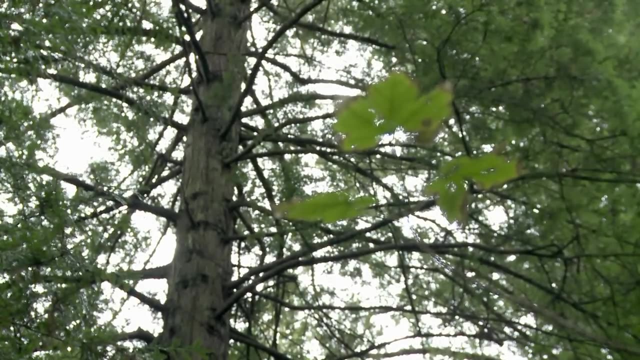 but it shows you how lignin can actually be changed in its properties. The quest to create plastic from wood continues, but another research group has managed to replace much plastic content with lignin In an extremely simple and ingenious way. They're adding wood fibre to plastics to act as reinforcement. This cuts down on the petrochemicals. 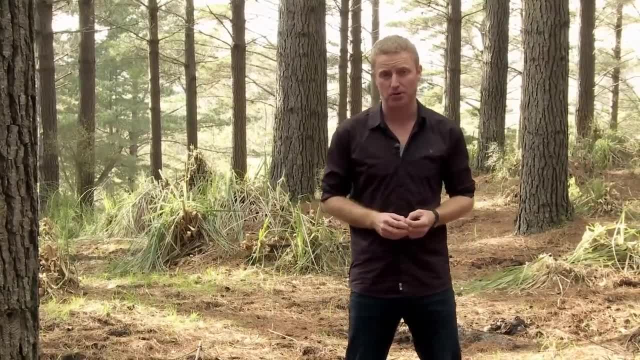 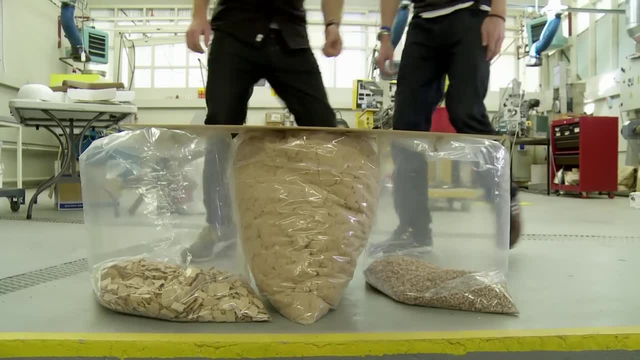 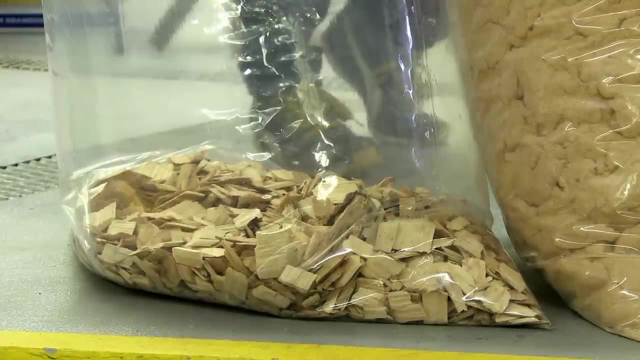 used and, crucially, fits into standard plastic processing, making it a project with huge global potential. Alright, so what's this stuff, Damien? It is the Scion wood pellet technology. We start with one and a half kg of wood chips and we transform that. 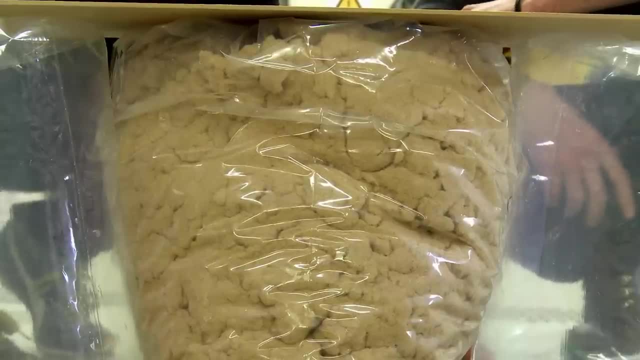 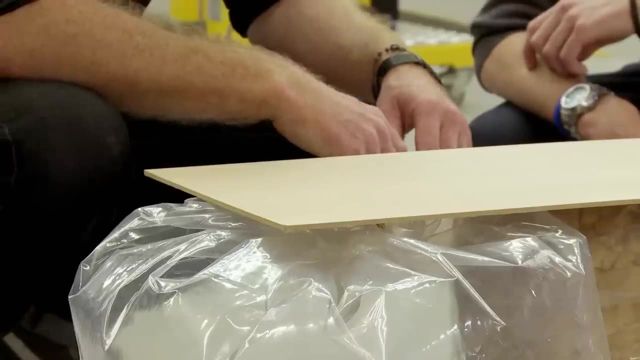 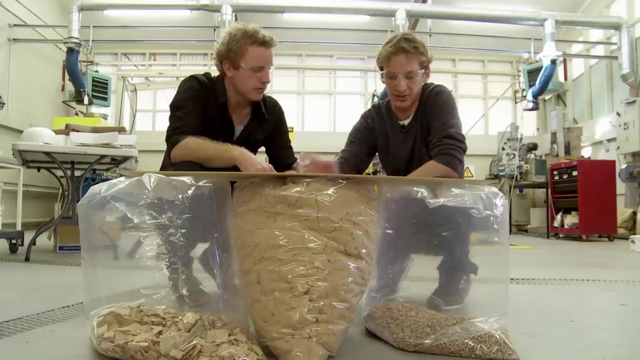 The problem is that there's no way for current equipment to use this messy, fluffy and highly flammable stuff, So Scion's smart invention is to create a binding agent that sticks the fibres back together but allows them to come apart again in plastic manufacture. 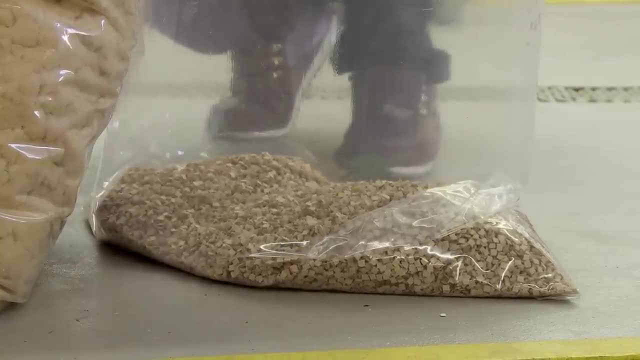 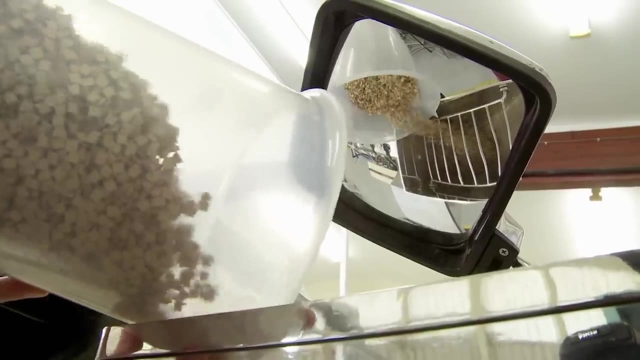 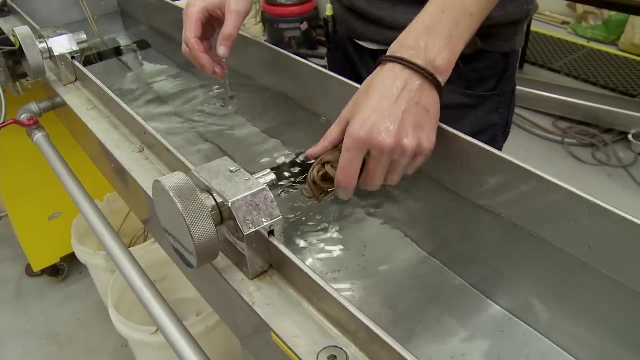 So this is the stuff that you're able to use. Yeah, it's dust free and it's free flowing, Really easy to handle and fit into plastic processing equipment. The wood pellets can now be combined with standard plastic. The secret binding agent releases the wood fibre to create wood reinforced plastic that can be used to make pretty much. 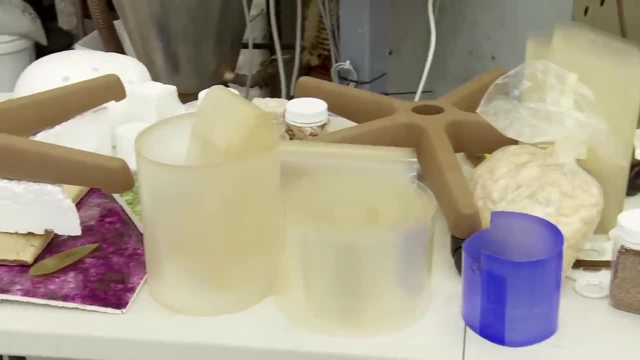 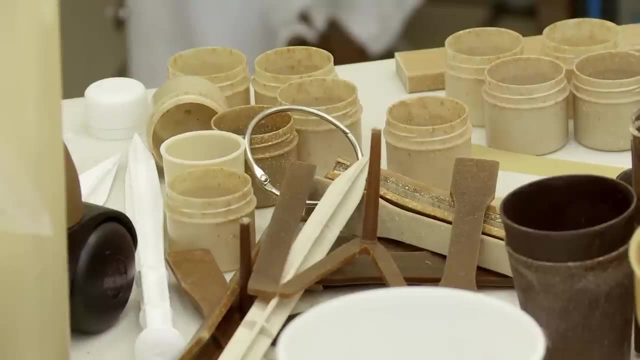 anything that plastic can. When you look at the amount of plastics that are used internationally, this could be a very large market indeed. Right now we've signed a licence with a company in Europe to start manufacture and they've got their first customer ready to start accepting some. 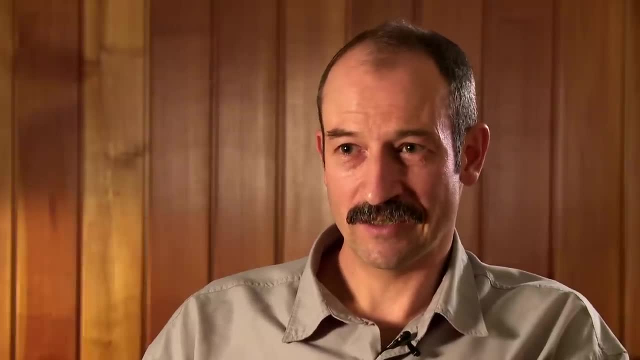 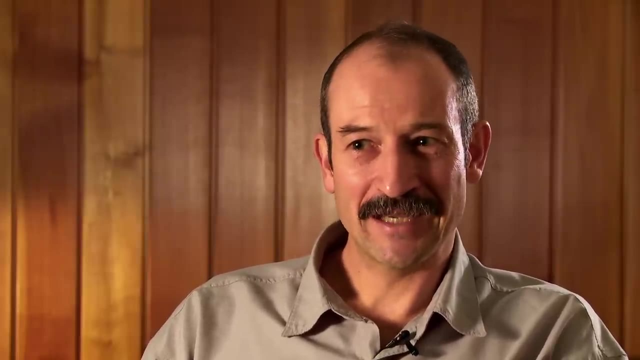 product. So when it finally comes to a point of that, we're ready to start manufacturing, We're ready to go. When it comes to a point of that final signature, it's almost surreal that it's been signed after the long process. So it took a few days to come to terms with the fact that, yes, it's. 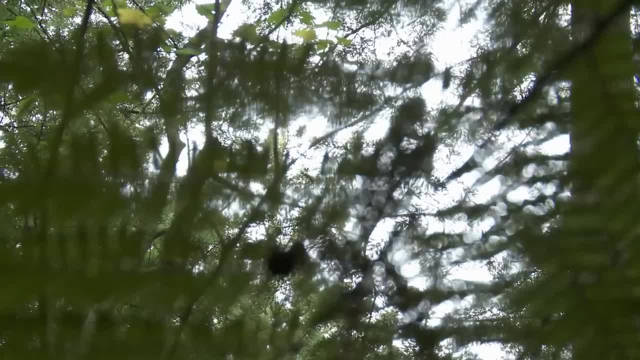 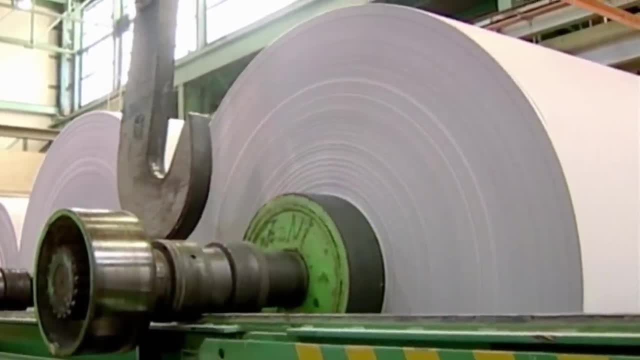 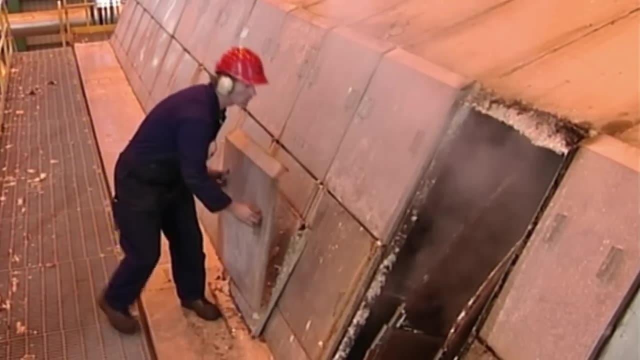 been signed and we've made a difference. Things are going to happen. Paper is an utterly enormous industry- About 300 million tonnes of it is produced globally every year- But it's an industry that uses vast amounts of plastic. It uses vast amounts of chemicals that are of environmental concern, And that's where 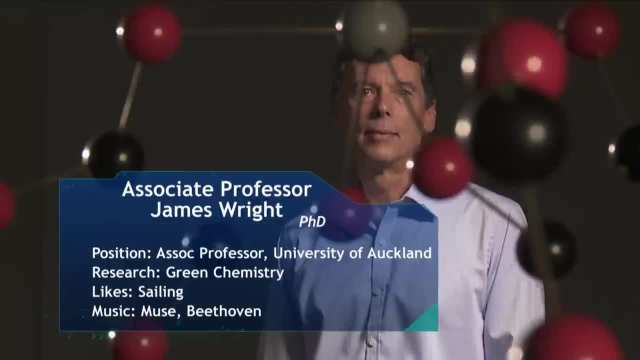 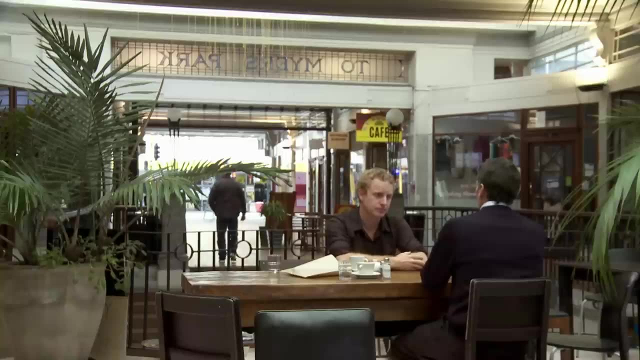 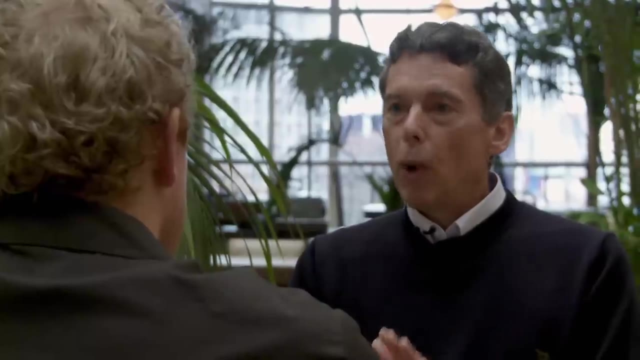 James Wright comes in. He's trying to find a safer and cheaper way to bleach the paper that we produce. The wood fibre that you get is a brown colour, a little bit like this brown paper bag that we've got here, And if you want to make white paper, you then have to take that material. 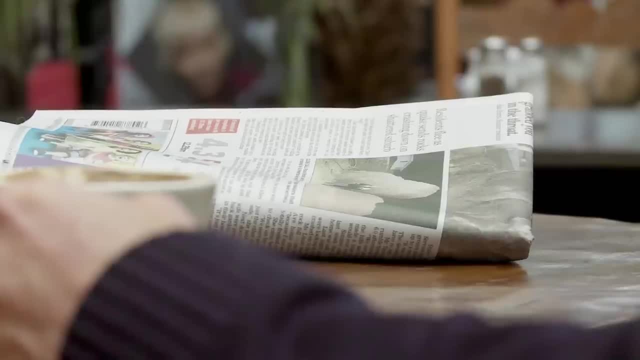 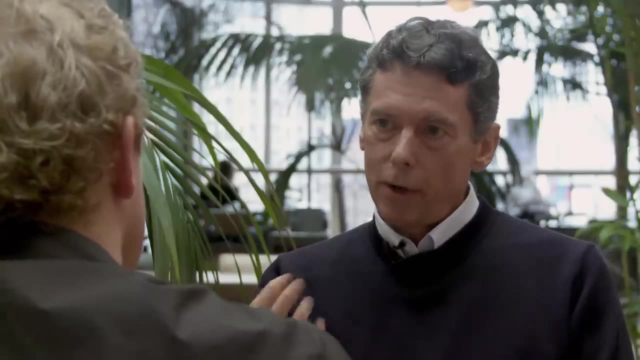 and chemically bleach it to make the paper white so that you get a good contrast. So you get a good contrast when you print on it. What kind of chemicals are used in that process? They use very strong oxidising agents, And oxidising agents are compounds that add oxygen. 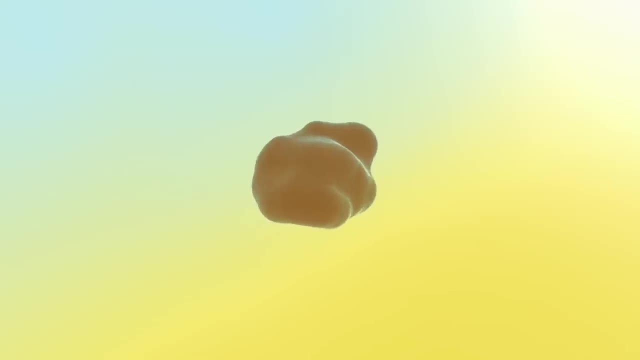 to molecules. The brown colour comes from the lignin molecules left in the paper In order to bleach this. an oxygen atom breaks off a small part of the lignin and miraculously gets rid of the brown colour. The only problem is that the chemical mostly used is chlorine based. 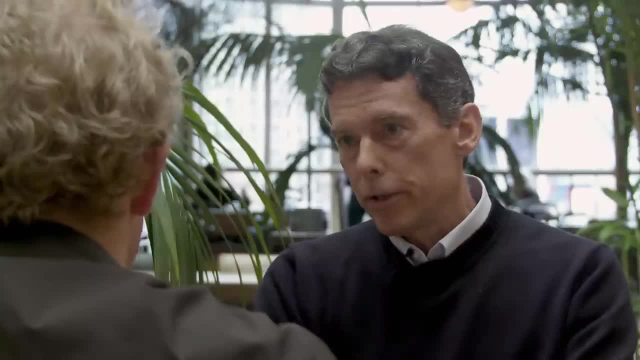 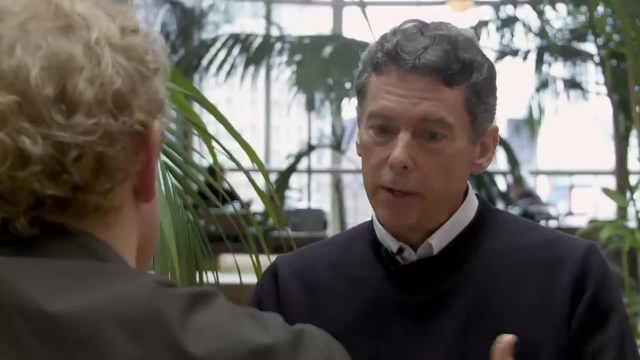 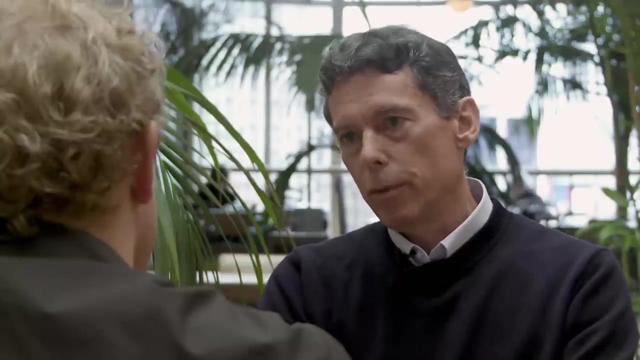 Chlorine's not the nicest of things though, is it? No, it's not, The reason being that in that process, you form what's called organochlorines, And these are very harmful materials generally. They're not materials that you want to release. 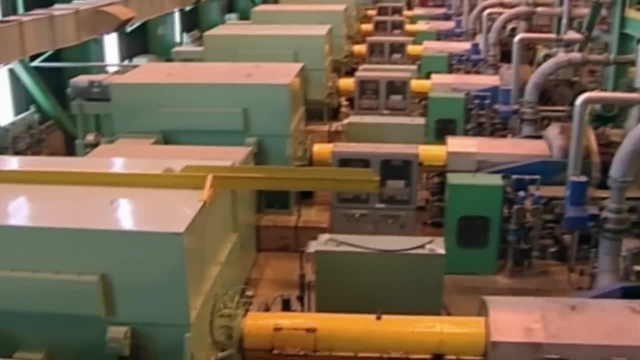 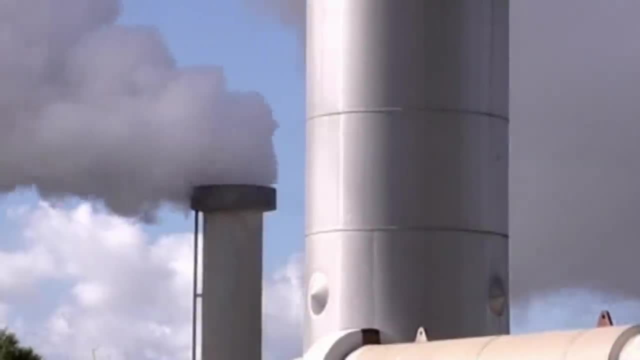 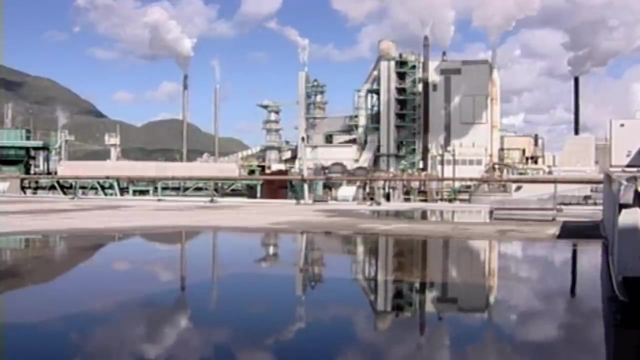 into the environment if you could avoid it. Processing these controversial chlorines is a long and expensive procedure, And there are still some environmental impacts. This has found a cleaner alternative that could revolutionise this gigantic industry. So what are you doing to try and invert this? 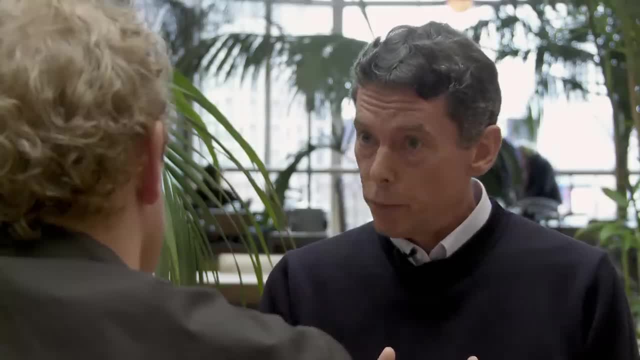 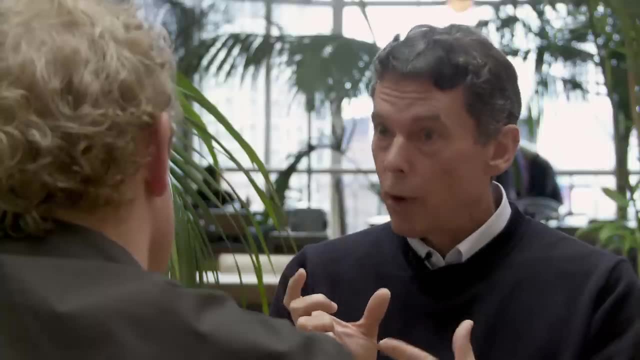 The oxidising agent that we're seeing if we can use is hydrogen peroxide, Just hydrogen peroxide. I mean that's quite a simple molecule. Hydrogen peroxide is a simple molecule, Just two oxygen atoms, two hydrogen atoms And 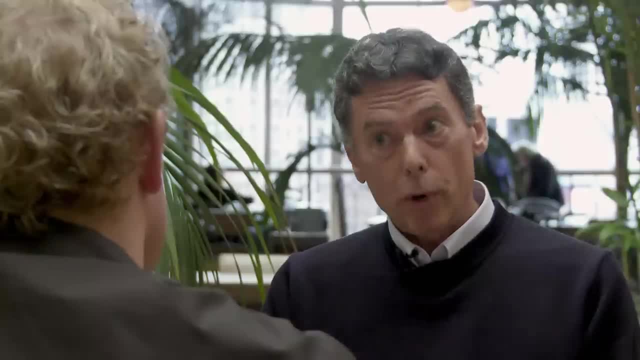 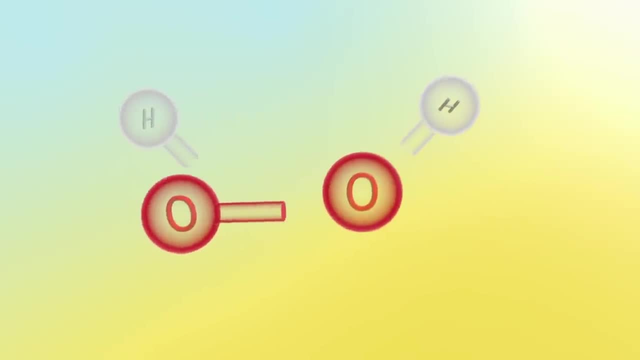 the beauty with hydrogen peroxide is that its breakdown products are just oxygen and water. That's great. That's safe, as So a tiny hydrogen peroxide…. Hydrogen peroxide gives away one oxygen atom to the bleaching process And we are left. 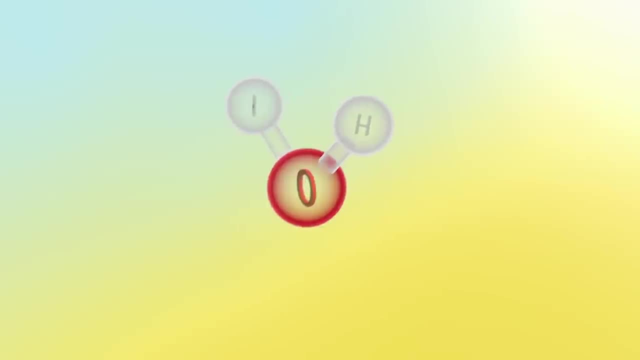 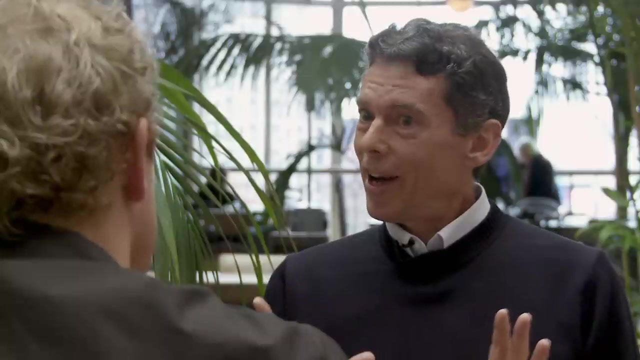 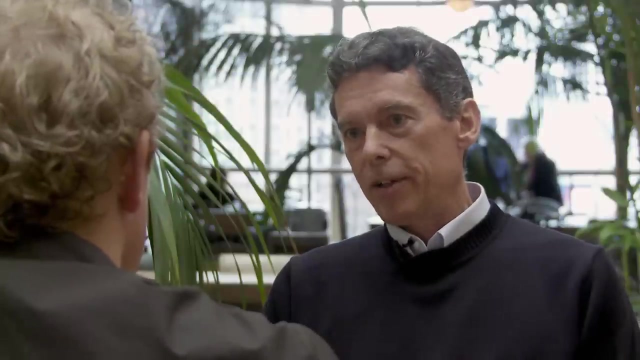 with H2O water, But why hasn't this beautiful reaction taken the place of chlorine already? The problem, though, with using hydrogen peroxide is that with these organic compounds, it reacts very sluggishly, very slowly, So you need to speed that up to make it effective. And 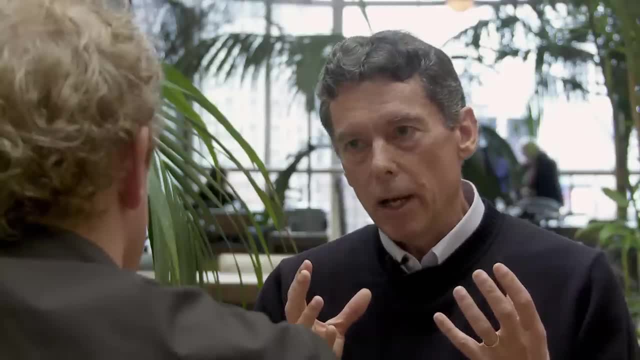 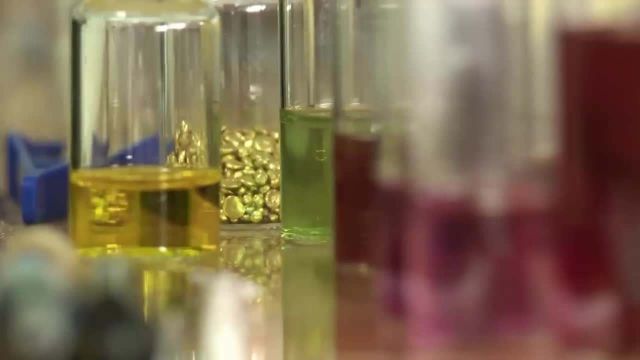 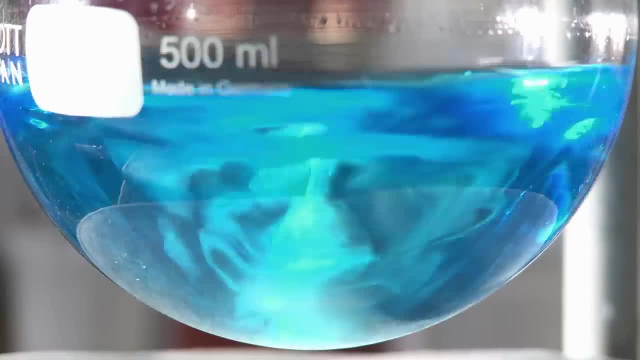 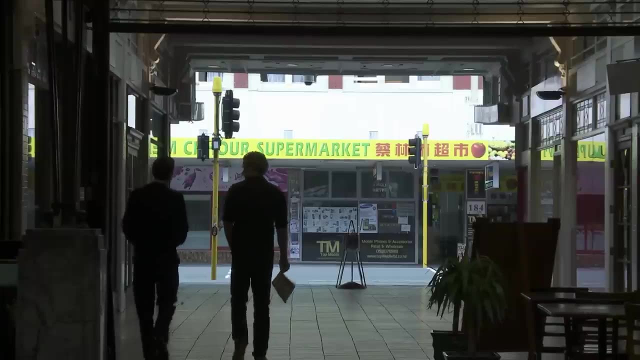 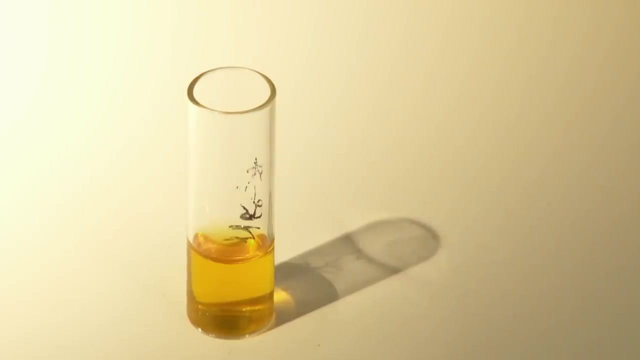 partnership without giving any of its own structure to the reaction. Finding a catalyst that would do this for hydrogen peroxide and lignin would be such a huge achievement that James has devoted almost two decades to the search And here it is. Let's see it in action. 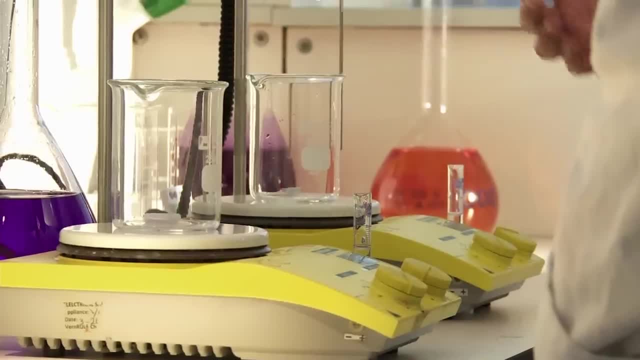 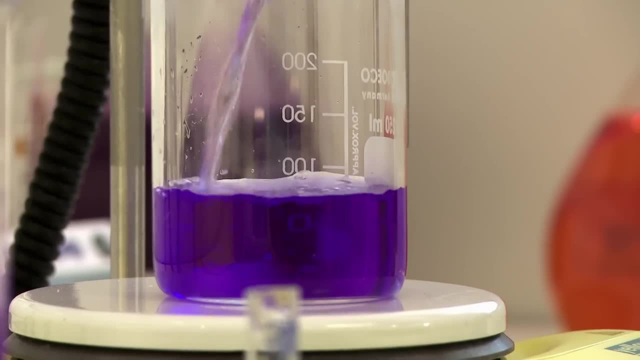 what we've got here is some, some purple dye, so we're going to oxidize this, that's right. so if you'd like to start off by pouring 100 mils of that into your beaker, all right. good, thank you, and i'll do the same. you turn the stirrer on. yeah, about 400 rpm that. 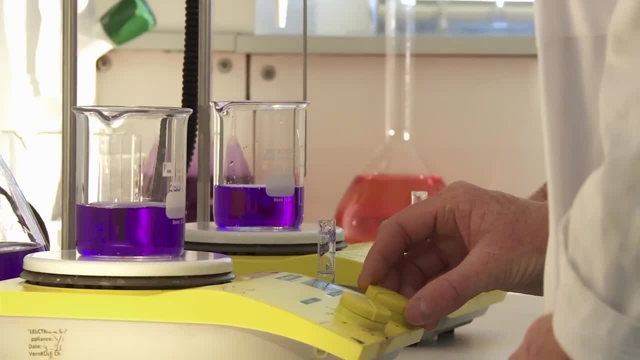 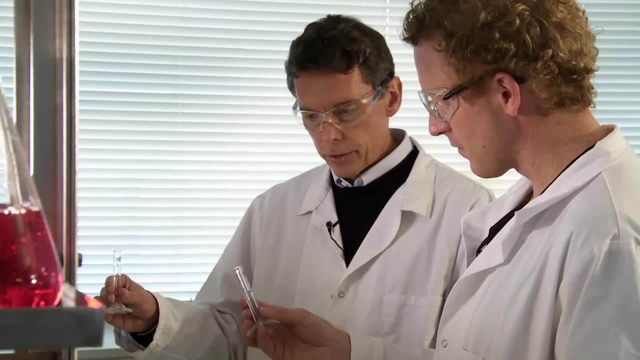 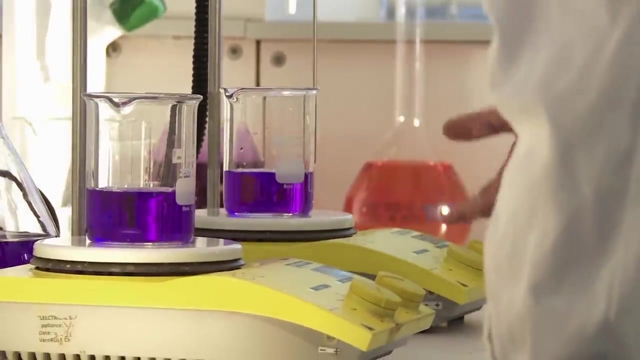 sounds perfect. come on, stirrer bar. yeah, there it goes 400. okay, so now, if you just take your hydrogen peroxide solution, we can add them at the same time, okay, okay, as you can see, nothing's happening. the color is still there, so it's going to go colorless when it's oxidized. that's correct. 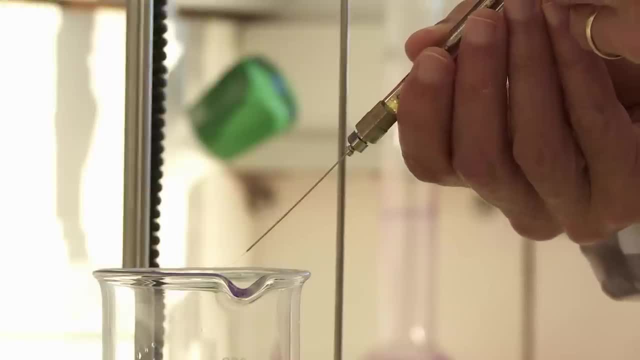 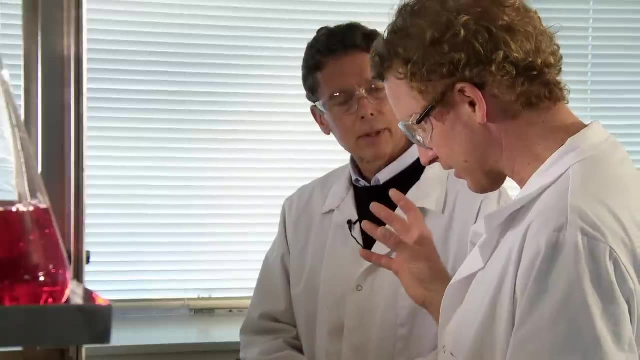 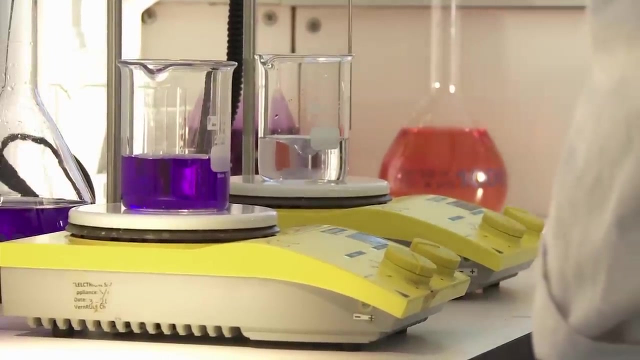 yeah, and now i'll take my solution and i'll add a catalyst to it and, ah, straight away, you can see that the color fades straight away. so the catalyst really is like facilitating that oxidation quite strongly, really speeding it up. yeah, as a chemist, i can see this is pretty impressive stuff, so i'm. 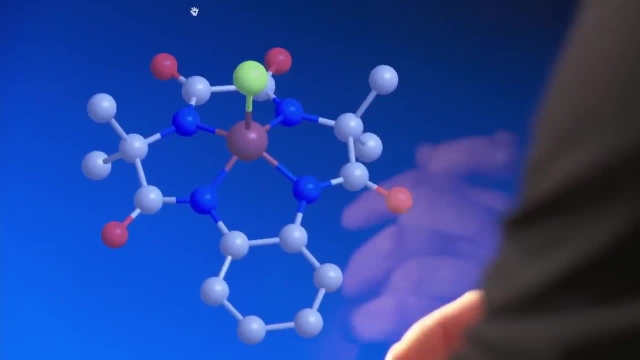 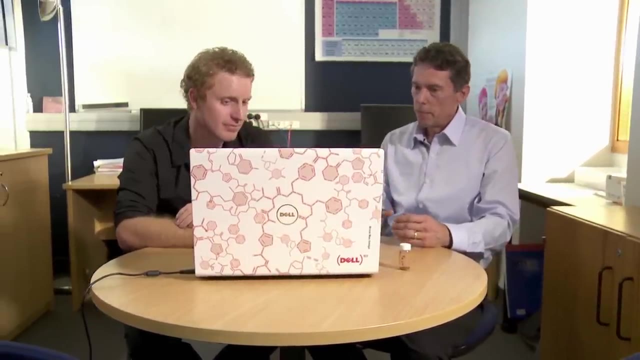 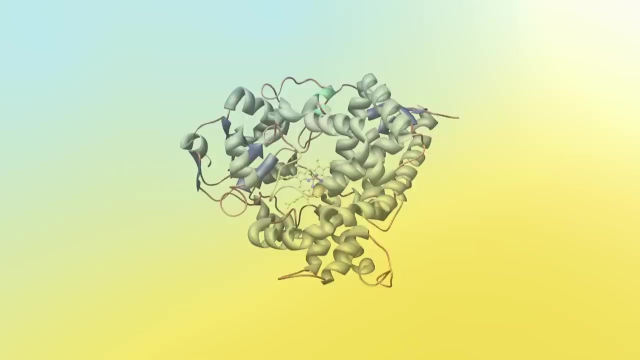 dying to see it. i can see this molecule, james, this is your complex. it's quite an elegant thing. well thanks. the original inspiration came from biology, so you could call this a bio-inspired design. james's inspiration came from a natural catalyst found in our own bloodstream. it's called cytochrome. 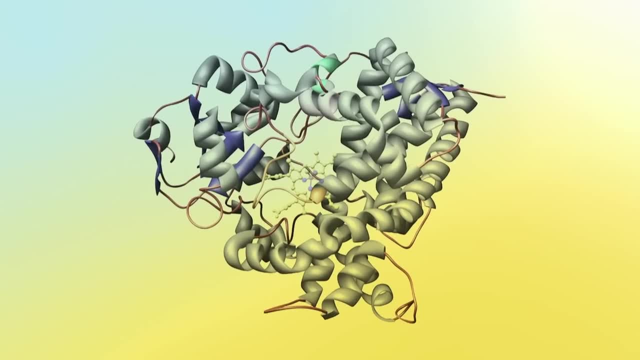 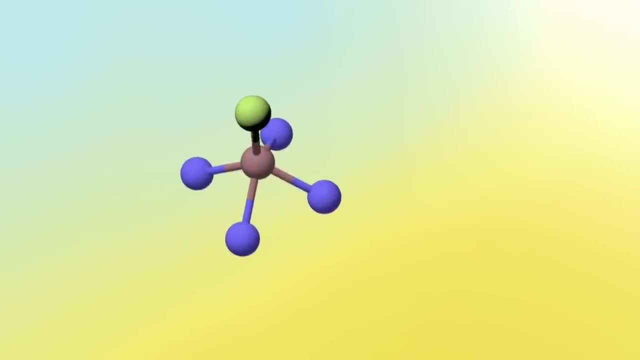 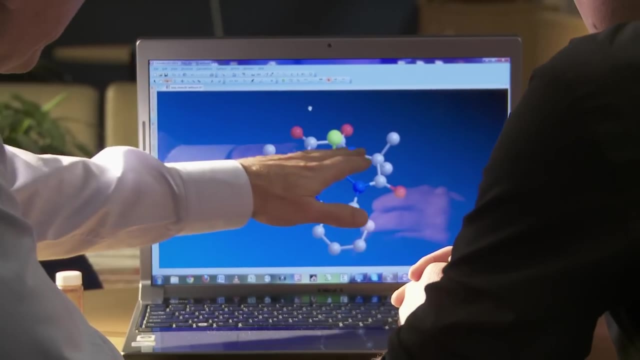 p450. as you can see, it is a ridiculously complex molecule. however, most of the action happens in a very small area. the central feature you'll see is the iron atom that's in the middle of the molecule here, and then, attached to that iron atom, are these chemical groups and we 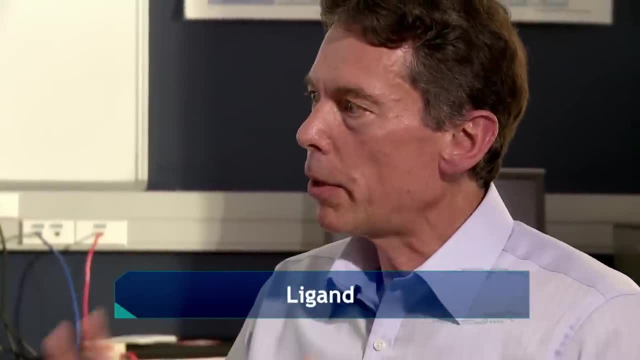 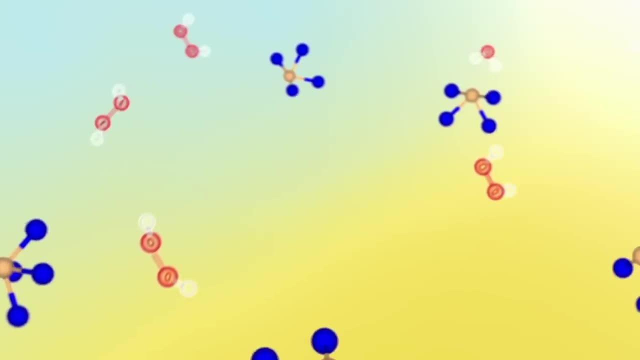 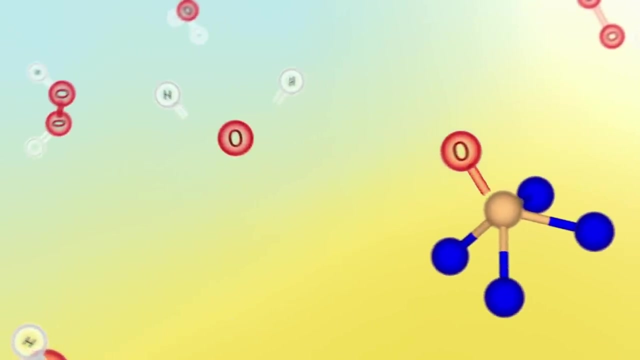 we call these ligands, and the role of the ligand is to modify the properties of the iron atom, basically making it a good catalyst. when hydrogen peroxide interacts with the catalyst, one oxygen atom is irresistibly drawn to the iron. however, this reaction gives the iron an extreme 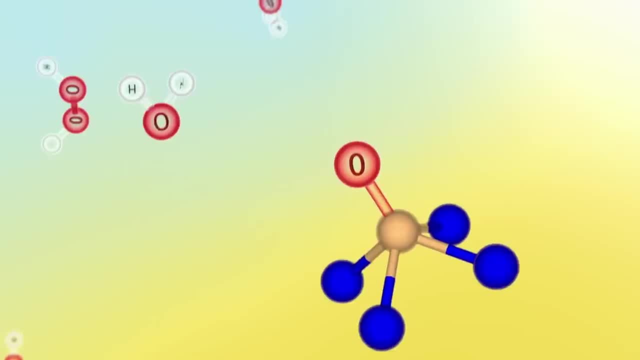 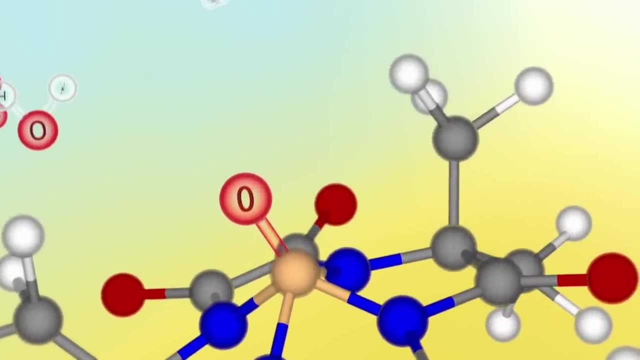 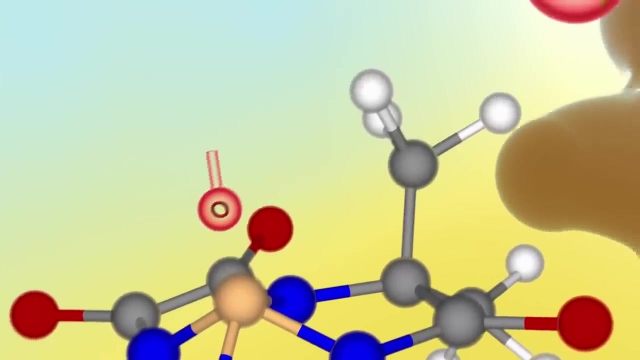 strong electrical charge. this would usually lead to the molecule destroying itself. but this is where the ligand comes in. it stabilizes the molecule and all that happens is that the iron transfers the highly reactive oxygen atom to a passing lignin molecule. then the process repeats. how? 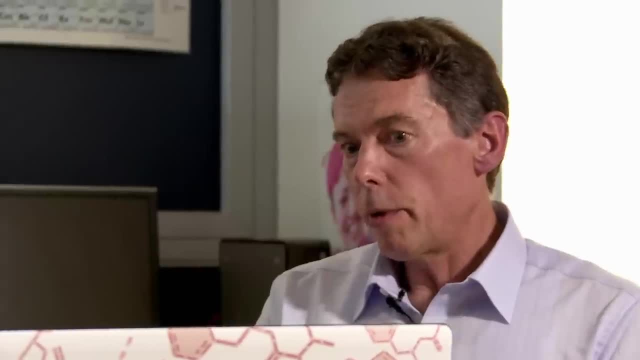 much of this. do you need to work? oh, incredibly small amounts. the the catalyst we have here is very, very active, so it's actually active for the molecule that we're dealing with here. so that's a very, very strong charge. this would usually lead to the molecule destroying itself, but this is where the 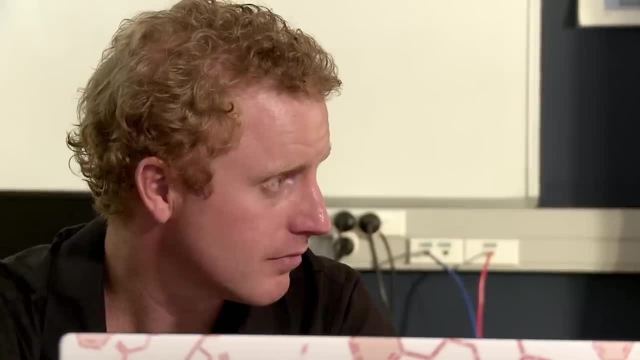 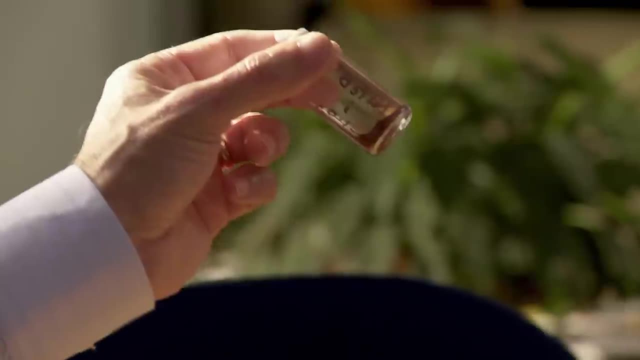 active at one micromolar concentration. One micromolar, One micromolar- That's nothing. That's really small. In fact, if you took this amount of catalyst and dissolved that in 5,000 litres of water, you would have a one micromolar solution. 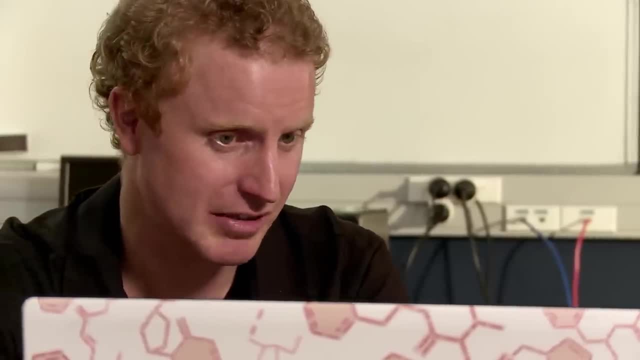 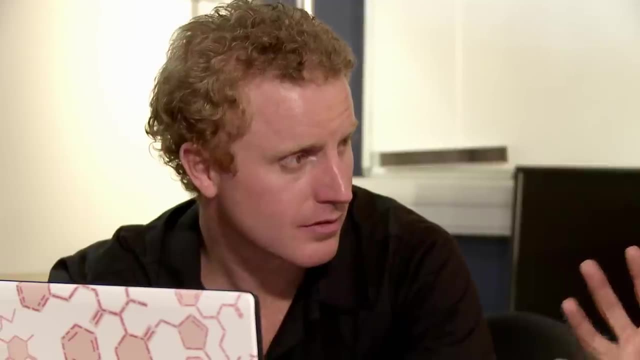 So that's really dilute. So when this goes into the environment, the effect is just negligible. Well, that's true. But there's an additional feature this molecule has, and that is, after maybe 30 minutes or one hour, it actually oxidises itself. And when that happens, it self-destructs and little bits of rust basically come out of the solution in an incredibly dilute form, Right? so if it does make it into the environment somehow, before it can affect anything out there, it's already attacked itself and become benign. 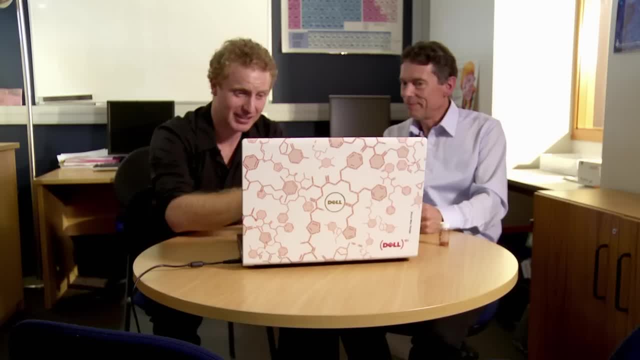 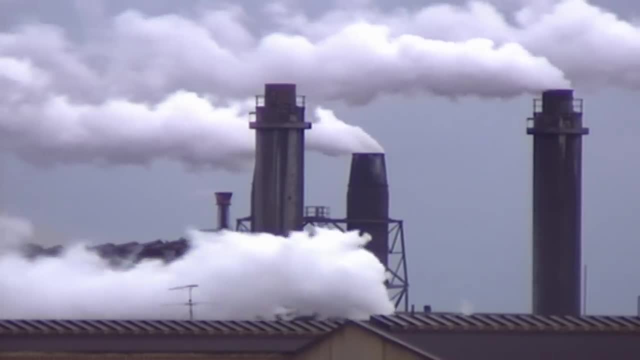 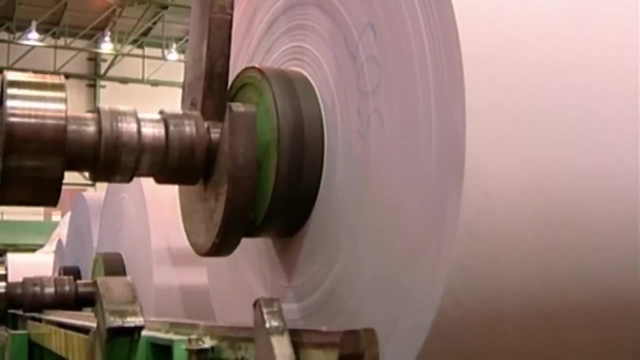 That's the design feature. That's brilliant. That's an elegant thing. The chemistry is just stunning, Thank you. Versions of this catalyst are currently being used in the US to process toxic waste and also Also in laundry powder, But the big prize is paper manufacturing. 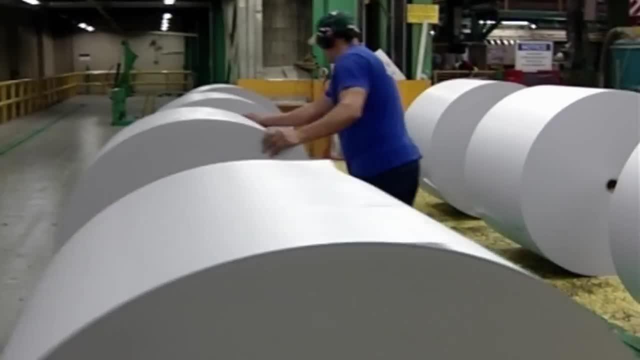 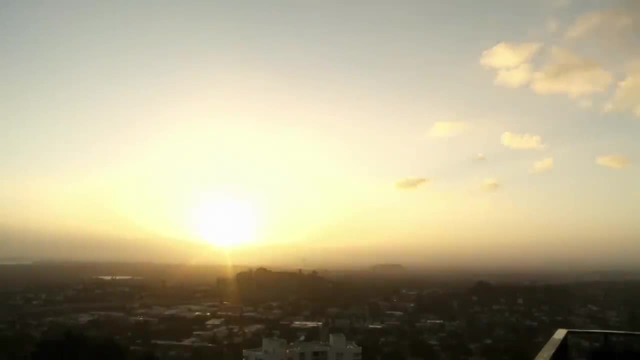 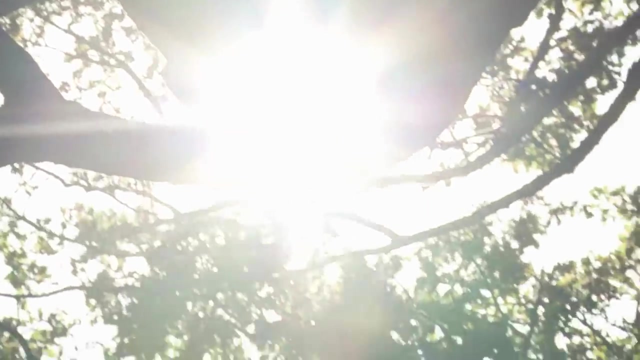 And James has been working with local companies to get it involved in paper bleaching here. Photosynthesis uses light from the sun to create electrical and chemical energy. It is the engine of life and is responsible for practically all of the food that every organism on the planet consumes. 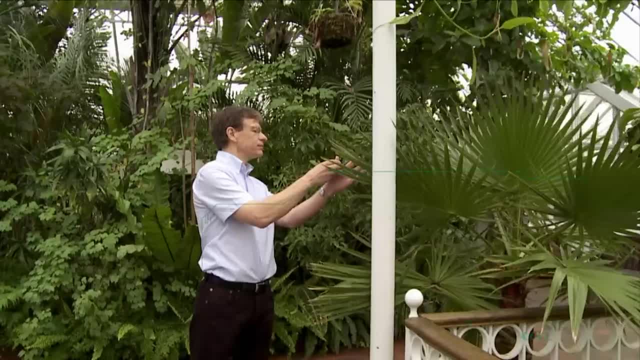 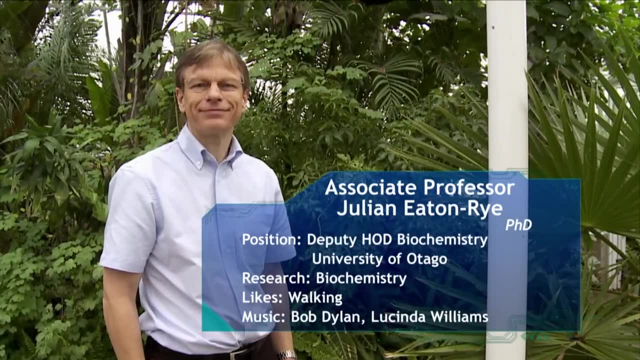 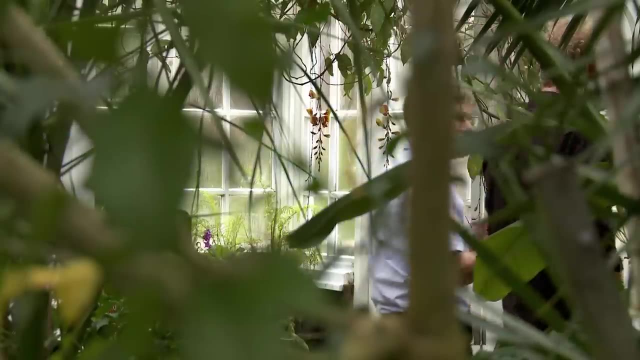 Replicating photosynthesis is the holy grail. That's why Julian Eaton-Rye is trying to unleash its incredible power. So, Julian, what got you into photosynthesis? I was fascinated by the way light and chemistry came together to create life. 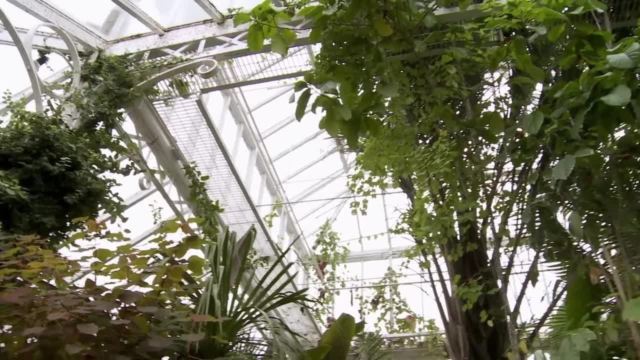 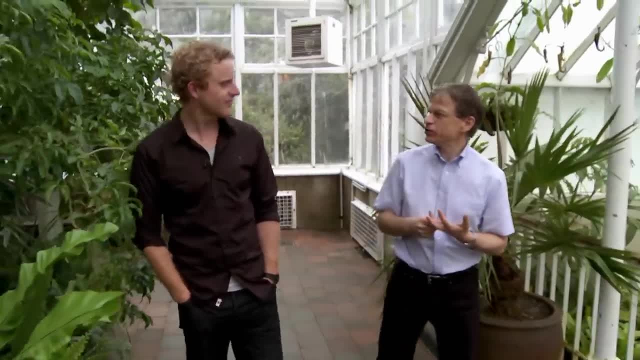 That was the first thing. It underpins everything that we recognise as life on the planet now, And that reaction has been described as the big bang. And that's the big bang in biology, Because that is where the oxygen of our atmosphere came from, somewhere about 2.5 billion years ago. 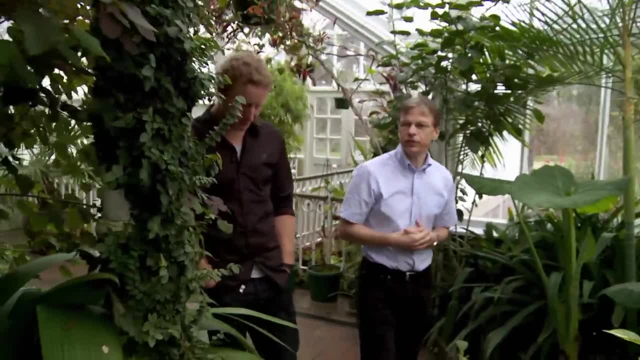 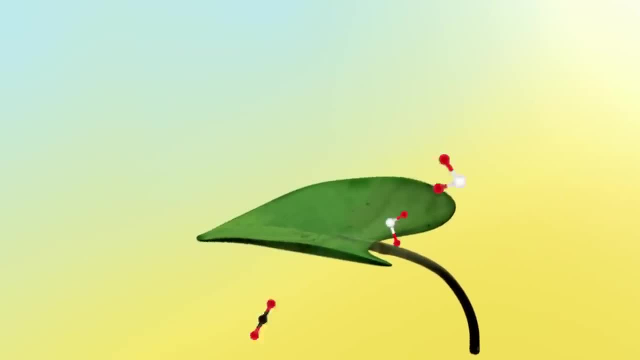 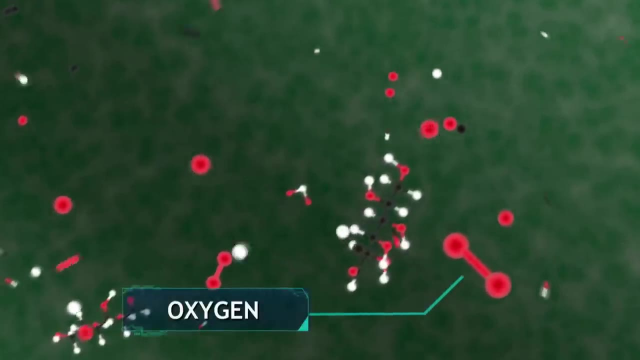 and transformed our world and allowed all this diversity of life that we see around us to develop. The basics of photosynthesis are that carbon dioxide and water go into the plant. Sunlight then comes in and rearranges these chemicals into oxygen and sugar, The part of this reaction that particularly fascinates Julian. 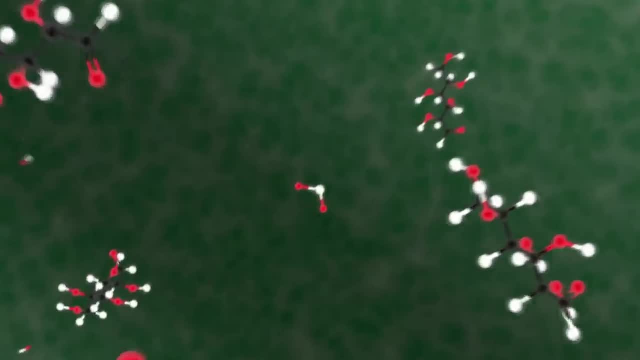 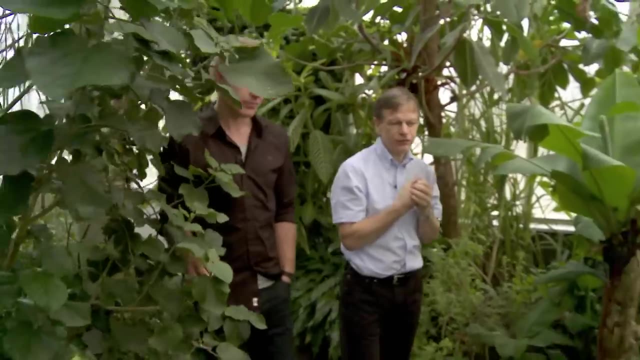 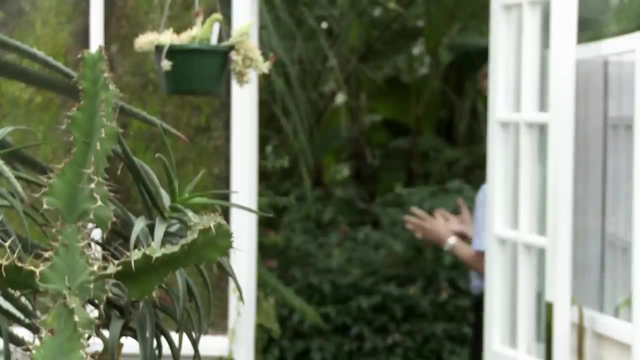 is how photosynthesis performs so efficiently. the amazing feat of splitting water. The reason that reaction is captivating is that if you want to split water, it isn't like boiling it in the kettle. It isn't steam you want, that's still water. 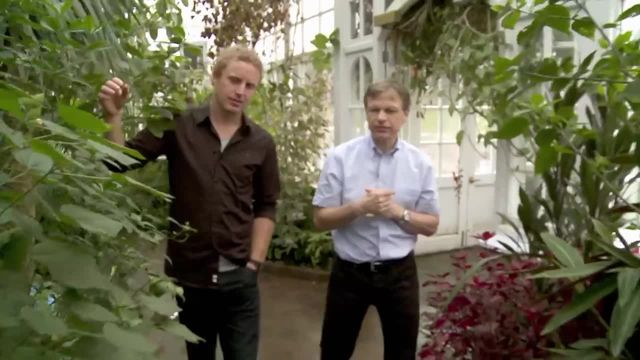 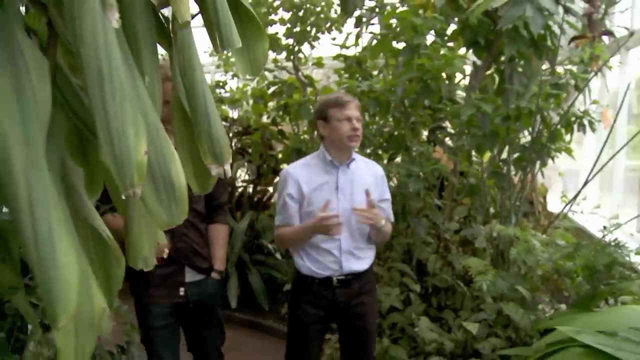 You want to split water and to do that you have to heat it to about 2,000 degrees, centigrade 2,000.. So this is separating the hydrogen from the oxygen. Yes, And here you are this morning in Dunedin. 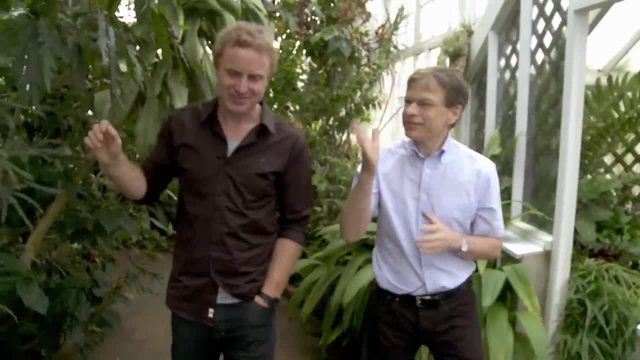 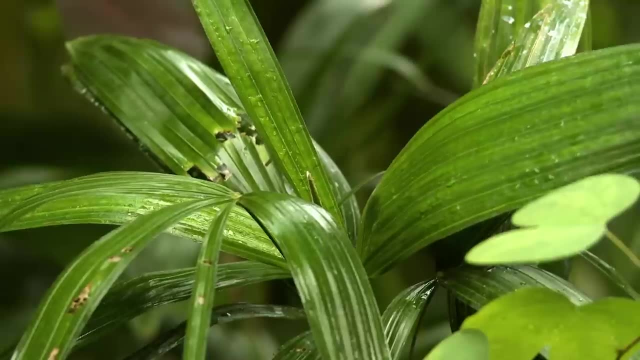 I don't know what it is. 3 degrees, 4 degrees, and the plants are splitting water. If you can understand how the plant does it, then you can take that and build synthetic molecules to mimic this process and you would have a system where you shine light and you split water. 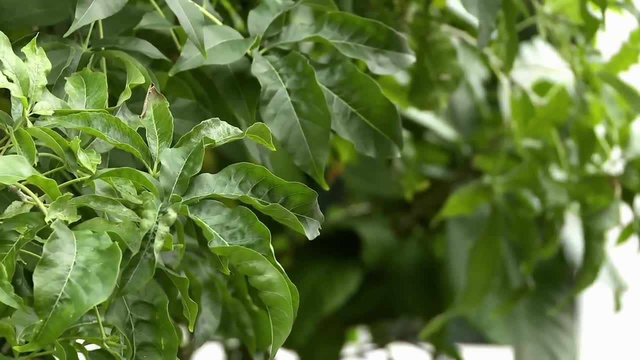 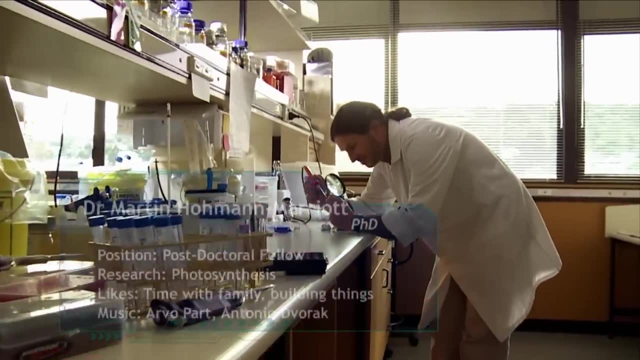 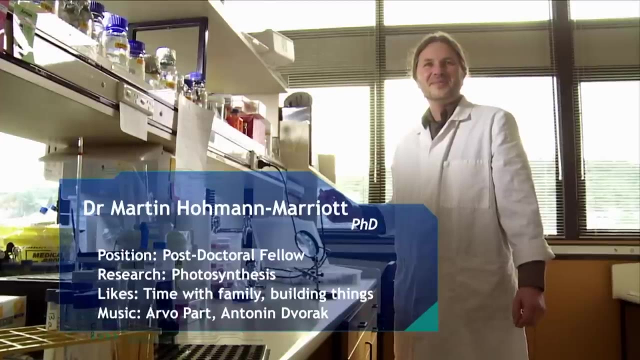 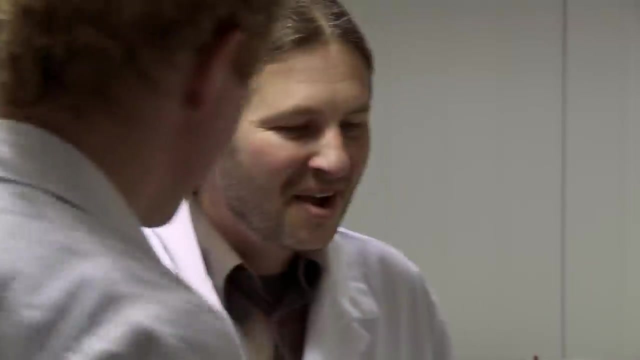 This is one of the biggest unsolved mysteries in global science, and it inspired Julian to start the Photosynthesis Research Group at Otago University, where Martin Homan Marriott is investigating some bacteria with world-changing potential. Ah wow, What happens in here? 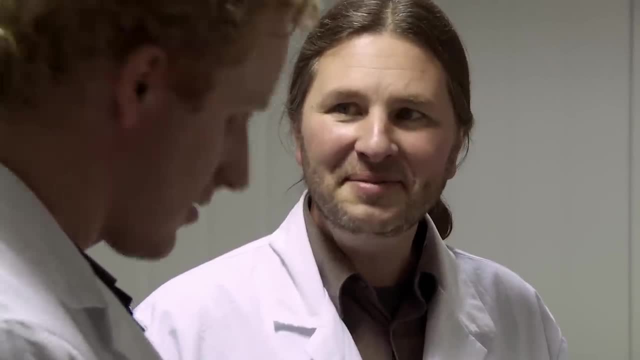 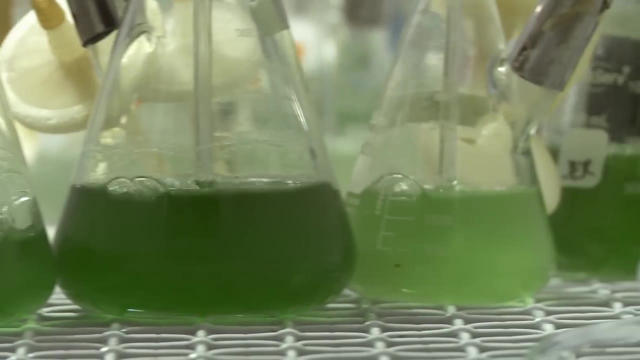 This is where we grow our bacteria. They are photosynthetic bacteria, So these are bacteria growing in these flasks. Yes, that's correct. The growth room uses artificial sunlight and perfect conditions to grow these single-celled organisms called cyanobacteria. 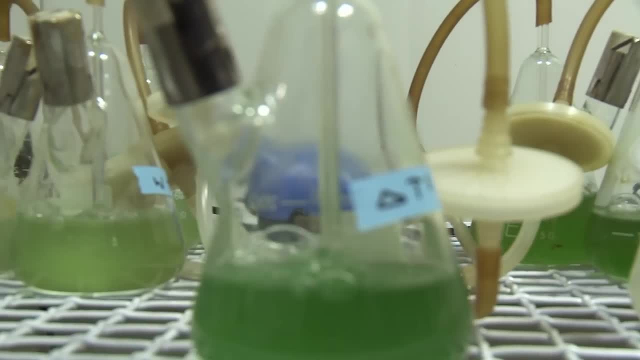 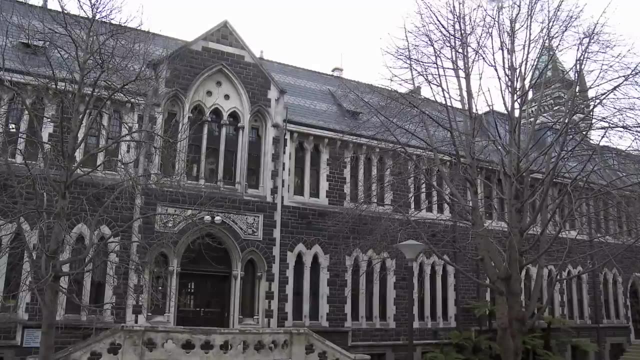 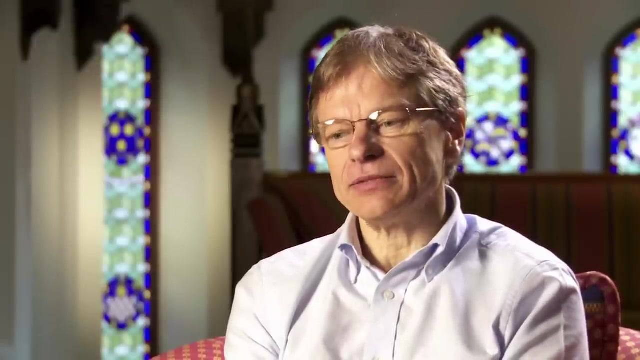 They are very efficient at gathering sunlight and splitting water. When water is split, it frees electrons. In other words it creates an electrical charge. Those electrons normally go into reacting with carbon dioxide to make sugar, But when you get excess electrons it actually becomes a problem for the cell. 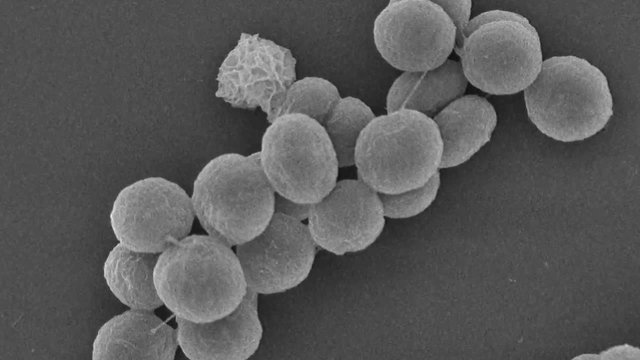 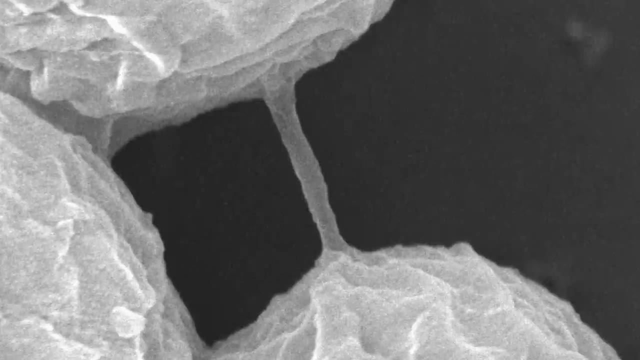 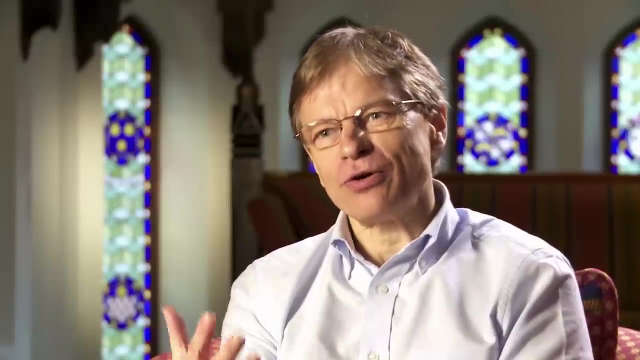 and it needs to jettison these excess electrons. So one thing we're working on is the possibility that you can actually use those excess electrons as a source of electricity and so have microbial communities that you shine light on and they make an electric current for you. So you're using bacteria to make electricity? Yeah, you can think of them as biological solar cells. Martin's research is at an early stage. However. he has already proved that he can take electricity from these bacteria, Right, Martin? what are we going to do here? 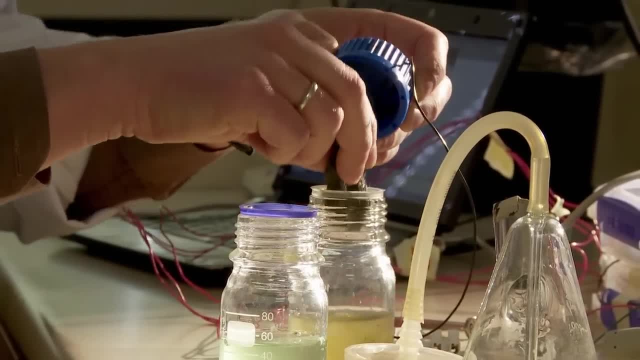 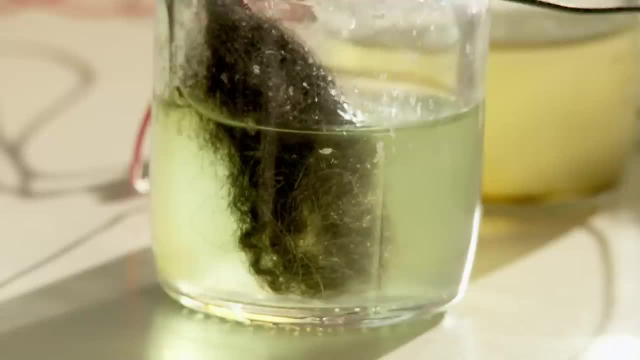 We're taking this rusty steel wool and transferring it here to our cyanobacteria, And over time this steel wool will turn from rusty into metallic again. And what's that telling you? That tells us that the bacteria are able to donate electrons to external sources. 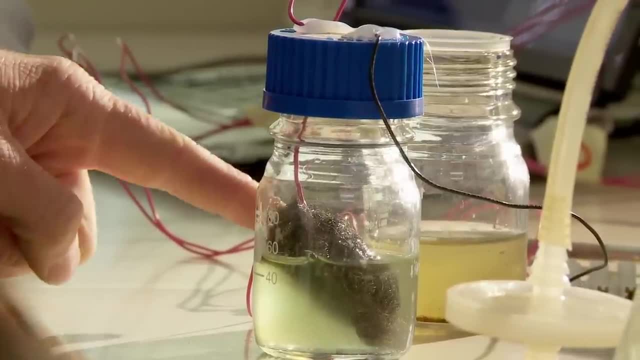 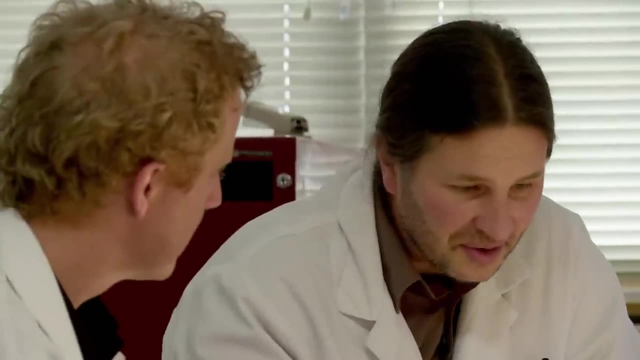 So seeing the rust disappear means that you're getting a charge from the bacteria. Yeah, it means these bacteria transfer electrons. And what does this mean for your research? It's a proof of concept at this stage that the potential applications are huge. 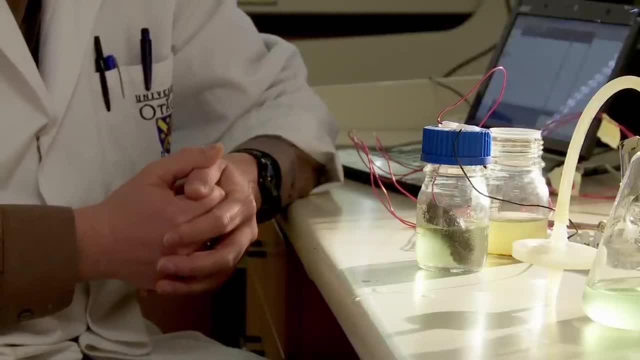 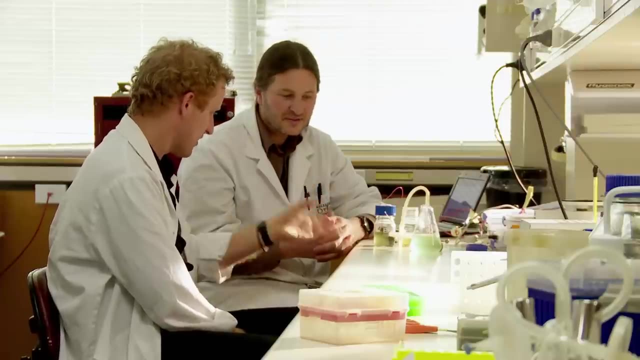 I mean, they can't be producing much electricity, though. No, at this time the scale is not huge, but the overall efficiency is very high. So this is proving that you can have a bacteria that acts as a solar cell. Yeah, that is the proof of concept here. 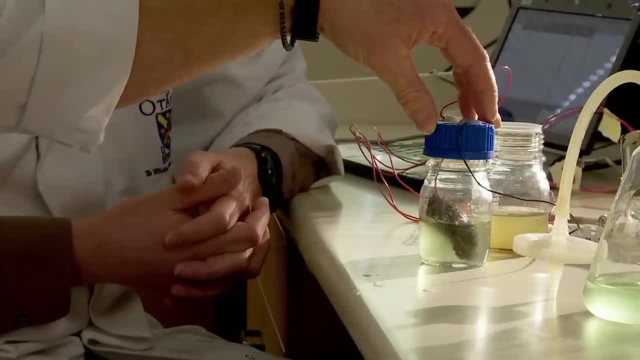 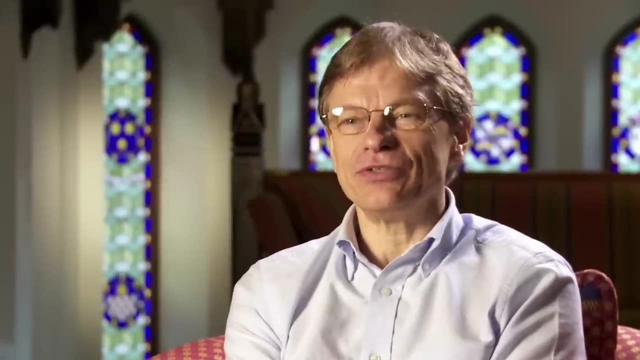 That's fascinating. At this time, the potential of the project is unknown. Of course, it will depend on how much current you can make, whether or not you can use it to turn the light on in your house. We'll wait and see. 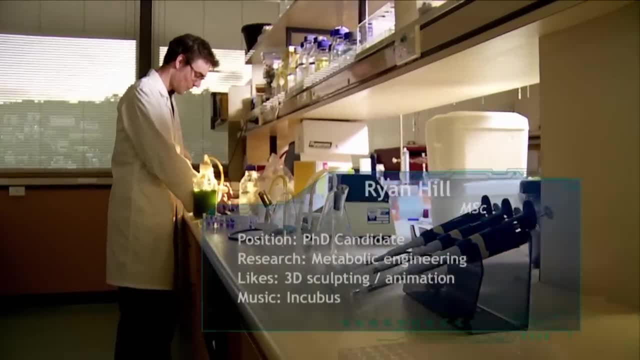 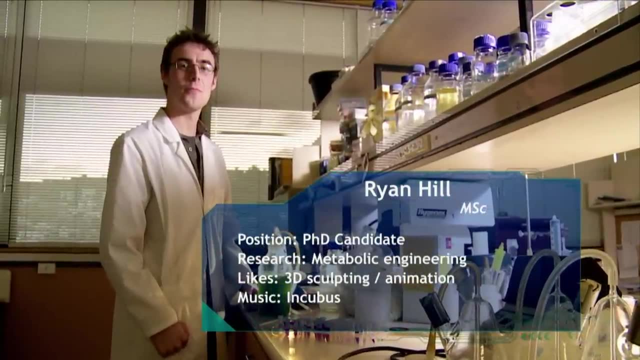 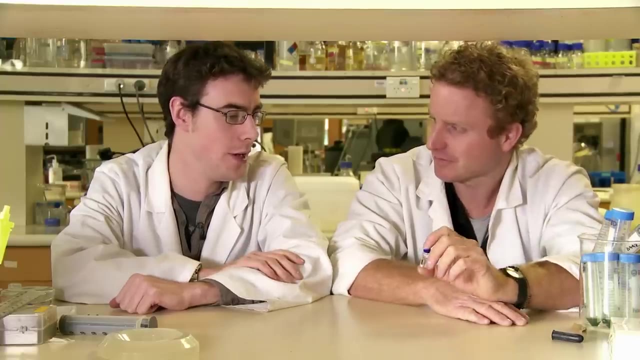 While Martin explores the electrical potential of bacteria, Ryan Hill is using the chemicals they create to find an answer to one of the planet's biggest problems. Ryan, what am I looking at here? That is butanol and water mix. Butanol is a pretty simple chemical. 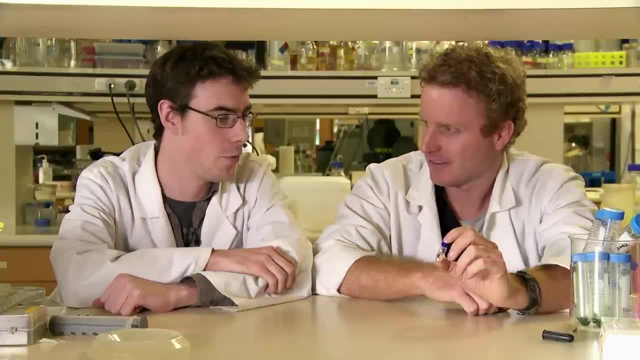 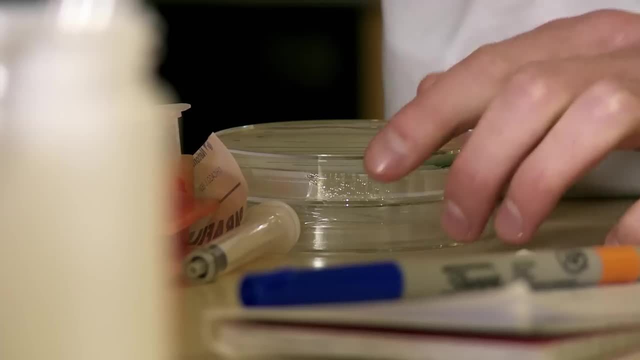 and what's special about this? That comes directly from a biological organism, Right? So how have you done that? What do you mean by that? Well, I've taken a bug. It's here. This is Sinicocystis. 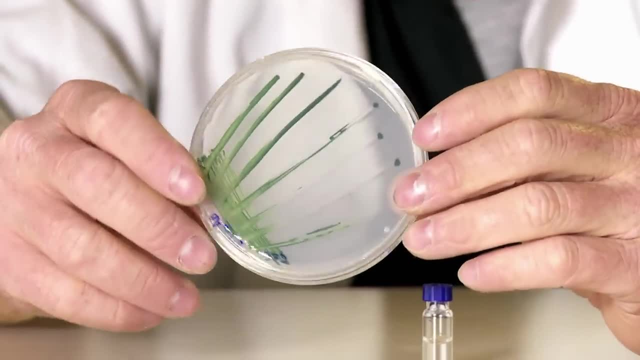 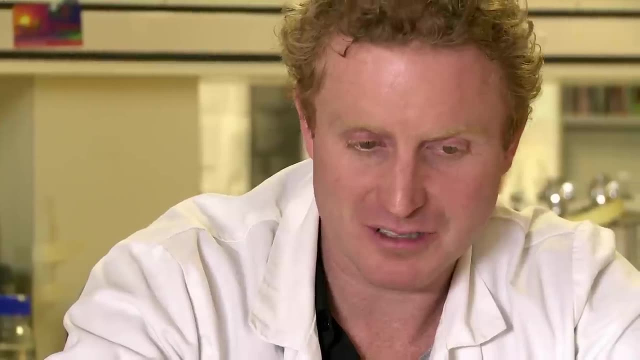 Now this does photosynthesis, which is what plants do, and it makes sugar from sunlight, And what I've done is basically reprogram it so that it takes that sugar and turns it into a fuel. So you're getting a direct fuel from this little guy here. 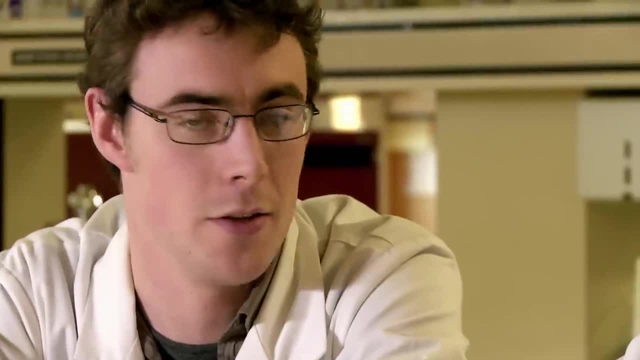 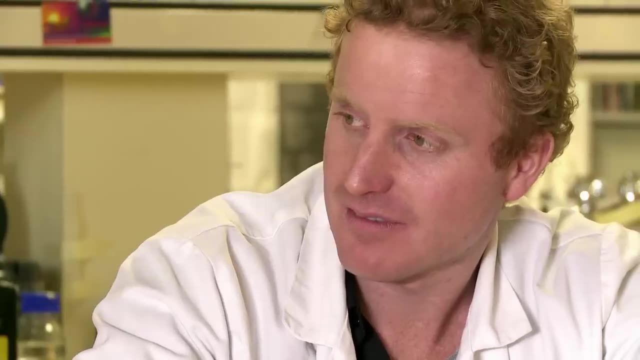 How are you doing that, Bacteria? they're machines, and the cool thing about them is that they're programmable machines. I basically write a program in a piece of DNA and I've put it into a biological version of a memory stick. 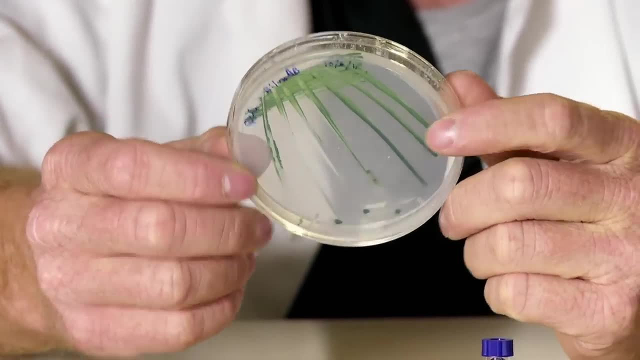 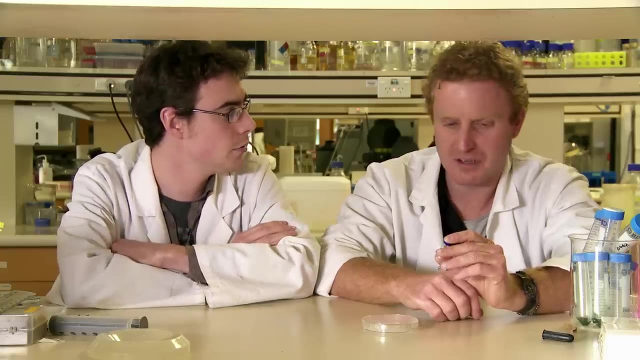 And you plug it into that guy and he installs it onto his genome and then he runs the program And that program tells it how to take sugar and turn it into butanol. So you've essentially made like a biological fuel factory. Yeah. 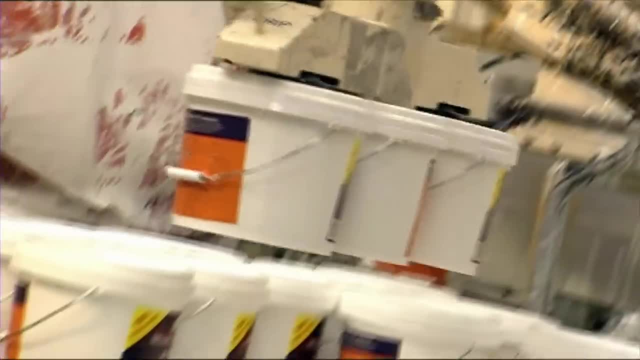 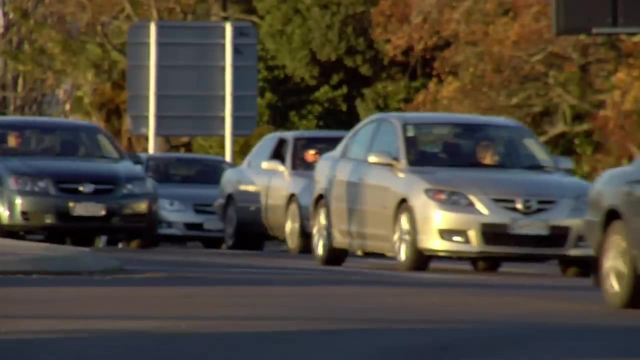 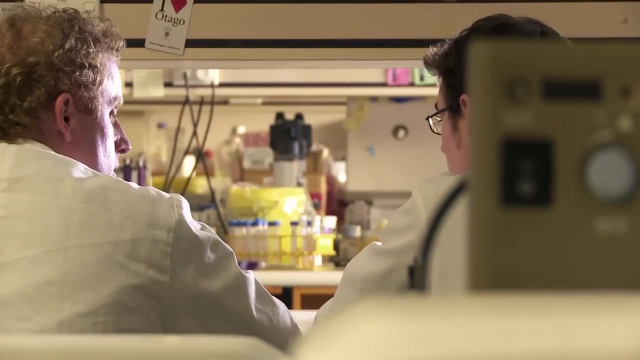 Butanol is a fossil fuel derivative that is used in vast quantities in such things as plastics and paints, But butanol is also a direct replacement for petrol. So this scientist in this lab may have the answer to the biggest problem facing our generation. Right now, we make very, very small amounts. 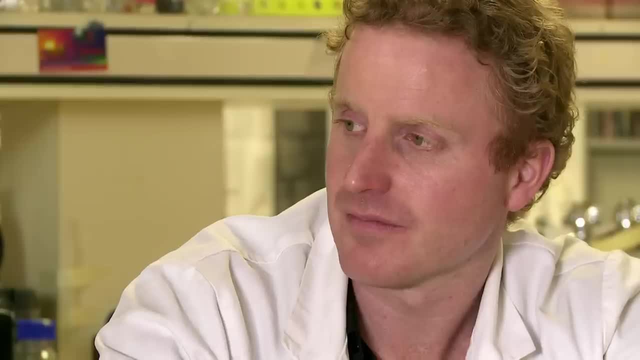 It's a proof of concept. We've got it to do it, but it needs to be at least 100,000 times better. So there's a bit of work ahead. There is a bit of work ahead, But you're confident. 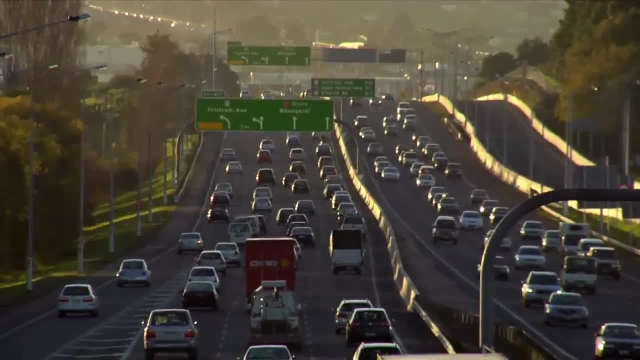 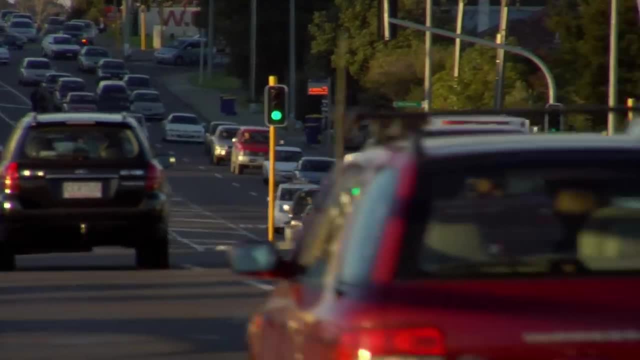 Yes, absolutely. If we can get it to that stage, it would be able to replace New Zealand's petrol. We use about 3.5 billion litres of petrol a year, and in order to do that, we need a land mass of about 0.1 to 1% of New Zealand. 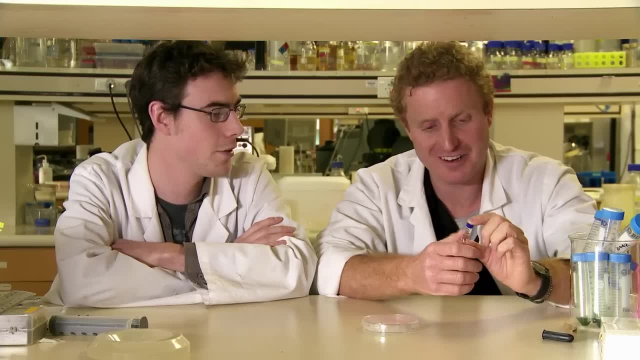 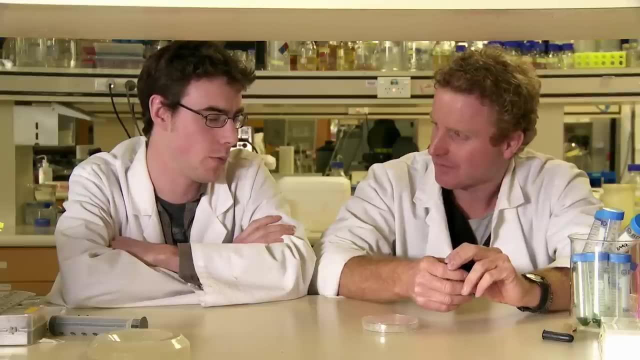 That's not much land at all. No, not really. That's really exciting. It's about one really big farm. Yeah, What about on like a global scale? To replace the world's petrol supply or meet current demands would require about 12% of Australia. 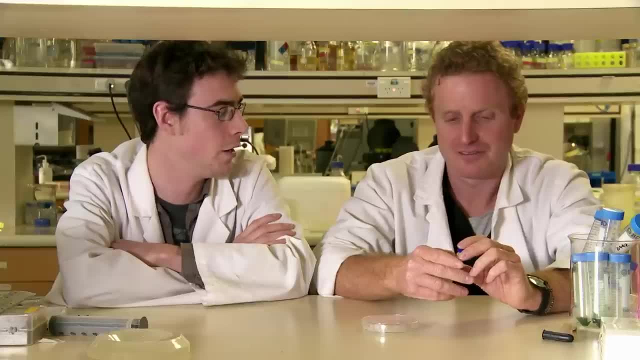 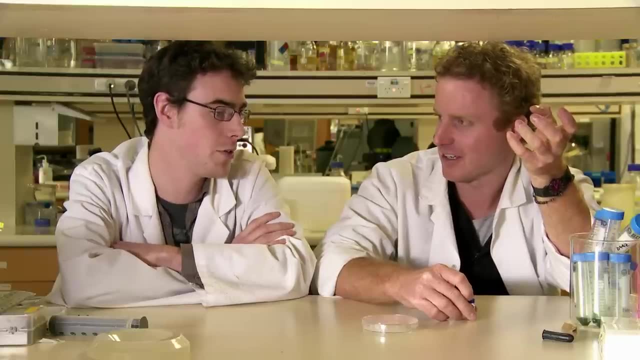 Which, again, is minimal. Yeah, and you can expand that, obviously, And I guess, being in Aussie, that's a lot of sunlight. Is that the idea there? Well, yeah, The vast majority of it's not. You can't farm it right.